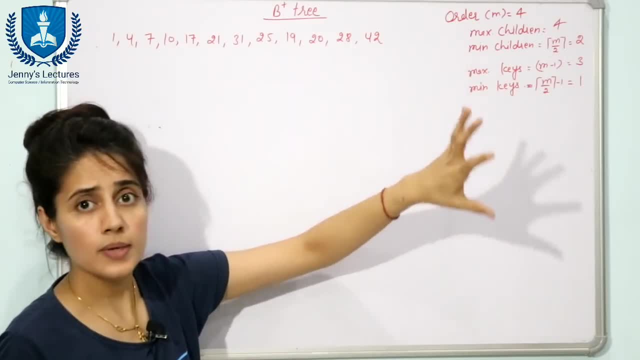 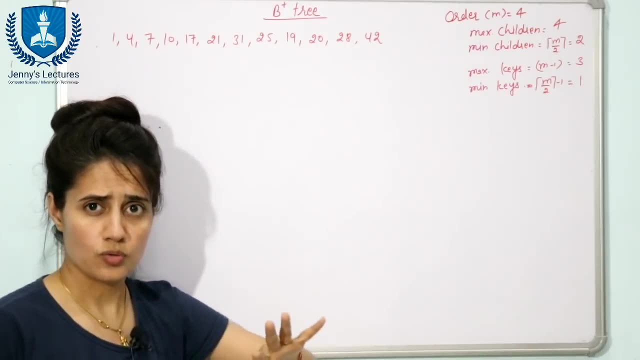 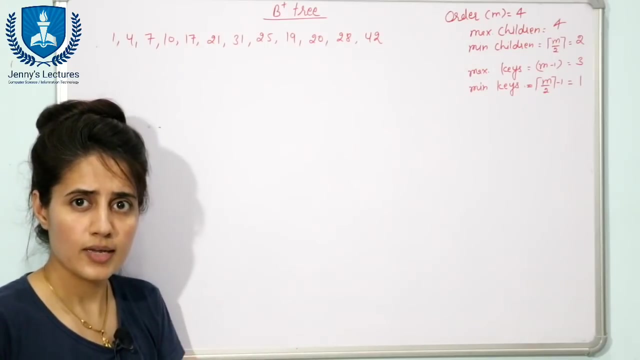 be 4. right minimum children can be 2, maximum keys can be 3 and minimum keys can be 1, except root node. See, these rules are not applied on root node. Root node can have maybe 2 children, root node can have 0 child. root node can have 1 key like that. Now the one main important property of 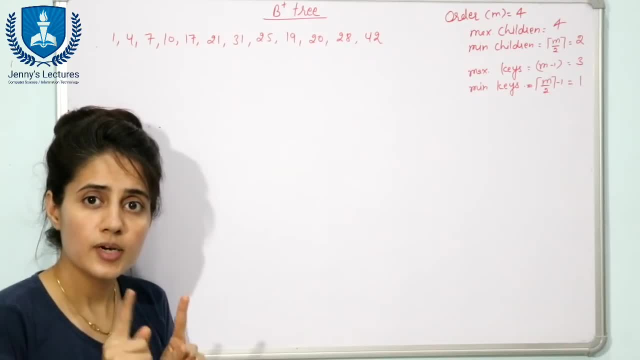 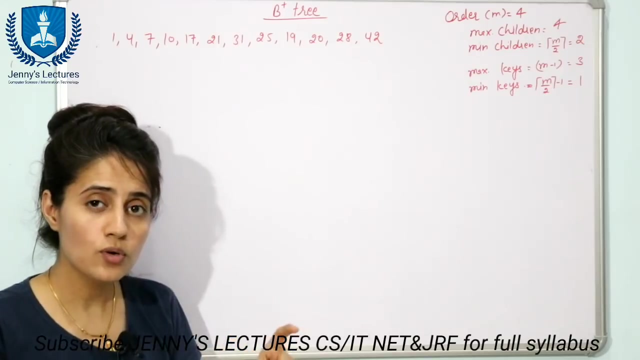 b plus tree is what In b plus tree the data. see this given data. this data is stored only in leaf nodes right and in b tree data is stored in leaf Leaf node as well as in internal nodes, but here the data is stored only in leaf node. 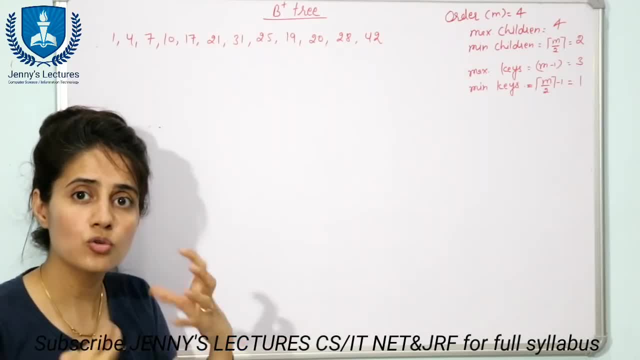 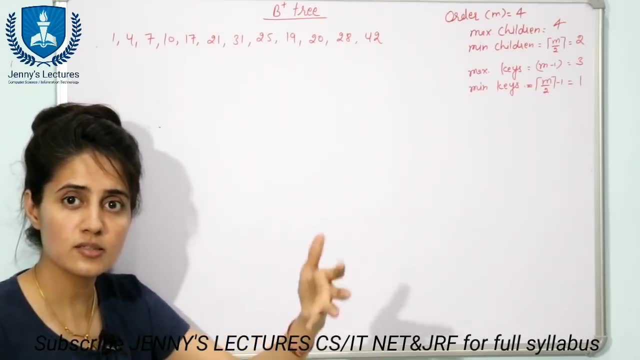 Now what is stored in internal nodes in b plus tree. Only the pointer so you can see the indexes, fine indexes to the data which is stored in the leaf node. Those indexes are stored in internal nodes. and second important point is the data which is present in leaf. 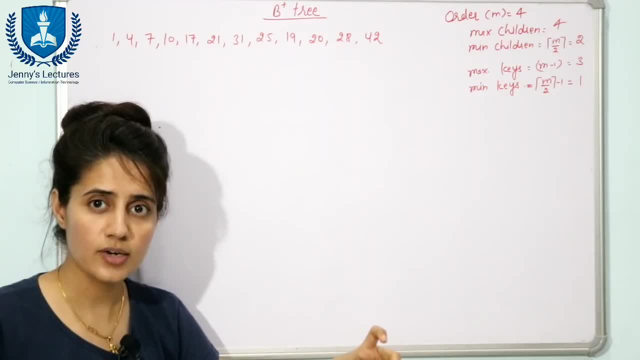 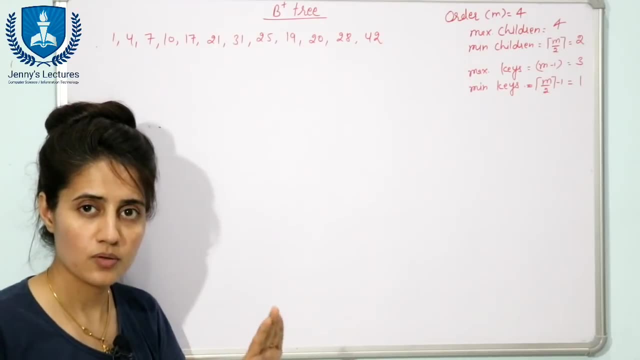 node. those data is present in a formal link list right. All the leaves are connected with a link with each other. I will show you how when we are creating a b plus tree with this example right. So these are the two main differences. I am going to make a proper video on b plus tree properties. 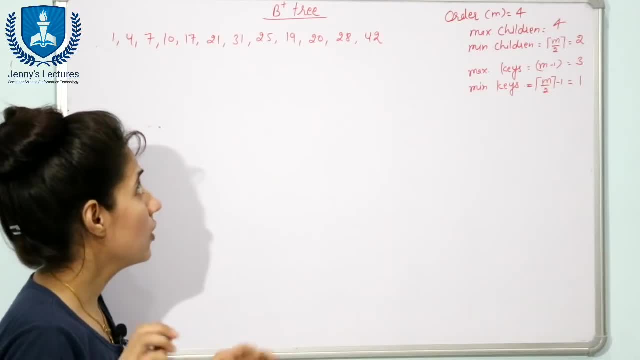 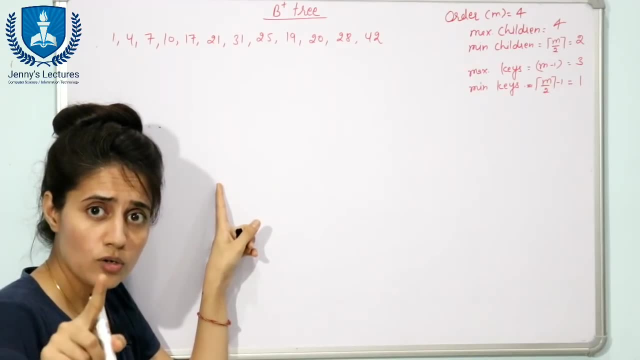 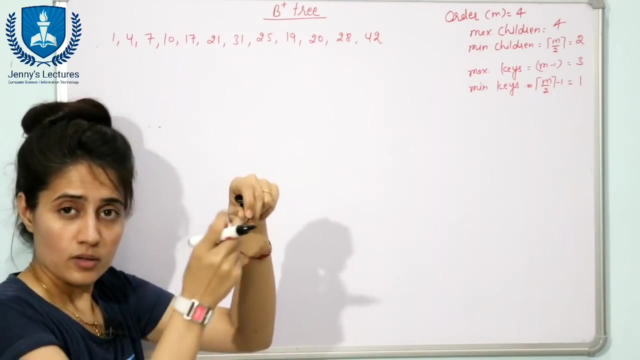 and how b plus tree are different from b tree. In this video I am going to tell you how data is to be inserted in b plus tree- right- See- and b plus tree- see. b tree is what it was: a generalization of bst binary search tree, So data in parent node. right, So the data. 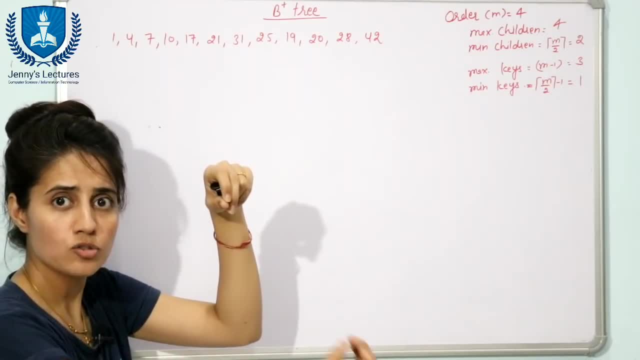 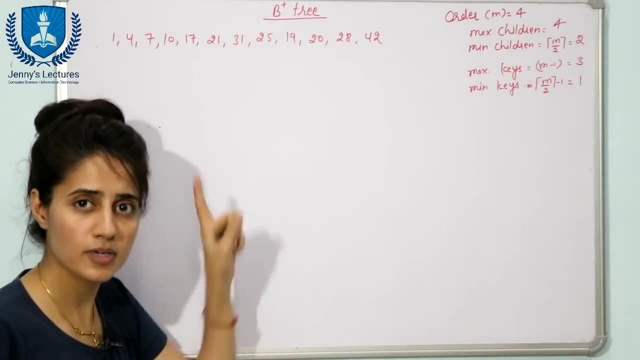 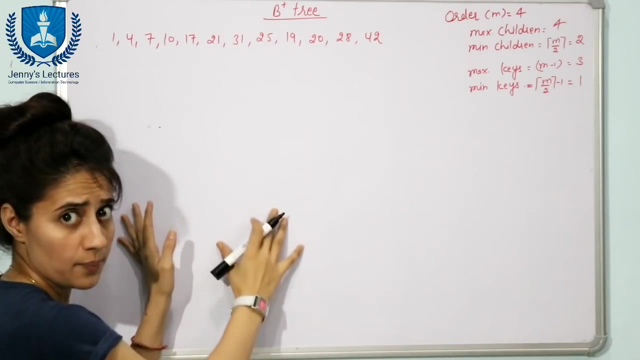 to the left of parent node Parent is always less than parent and data to the right of parent is always the greater than that parent. So that property is always. that property is also followed in b tree as well as in b plus tree. So now let us start See here. order is 4.. So initially, node trace there is 3 is empty. 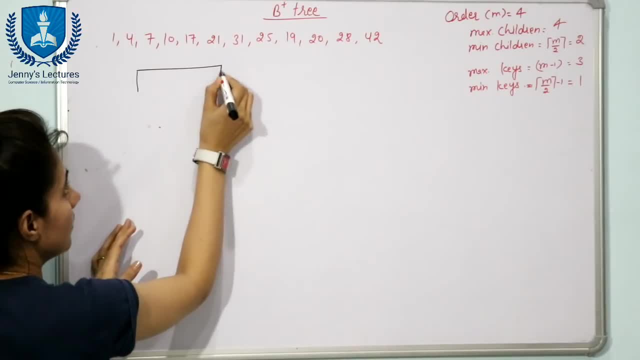 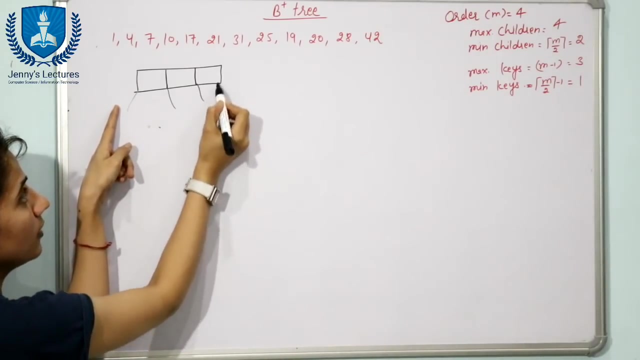 So we are going to construct a node- you can say right, and that node can have maximum how many keys? 3 keys, So that node can have maximum 1, 2, 3 keys And maximum children can be 1, 2, see 1, 2, 3 and 4.. So in between these 4 links only 3 keys. 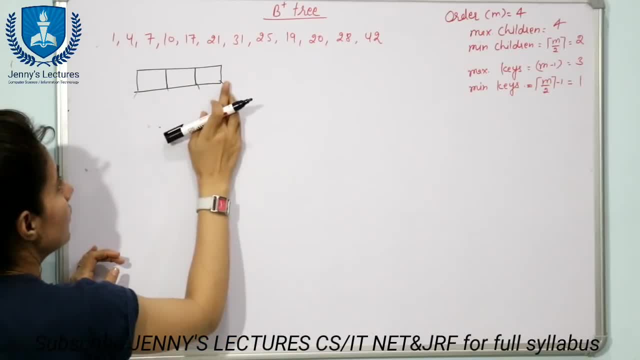 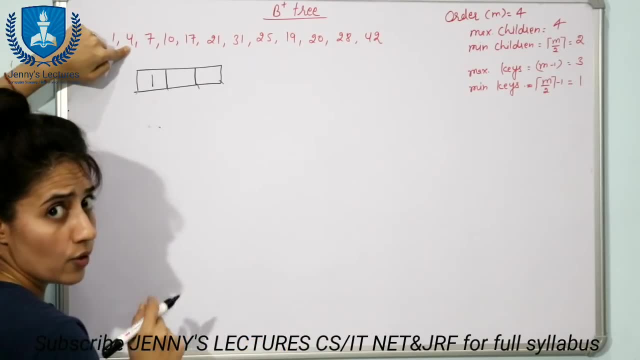 are possible, right. So now see first. first number is 1, insert 1.. So we can insert 1, right, So next. next is 4.. Now, where 4 is to be inserted, 4 is here. only one node is there, right So? 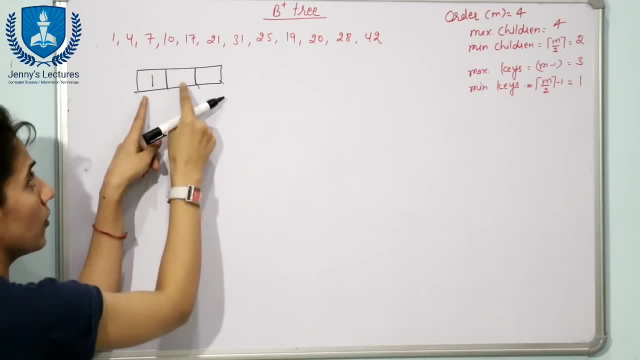 4 is greater than this 1, so 4 is to be inserted to the right of this 1.. So here we will leave 1 and we will insert 4.. Next is 7.. 7 is greater than 1. also greater than 4. also, Here we will. 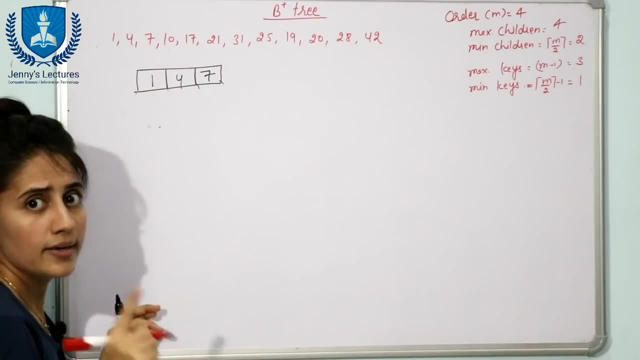 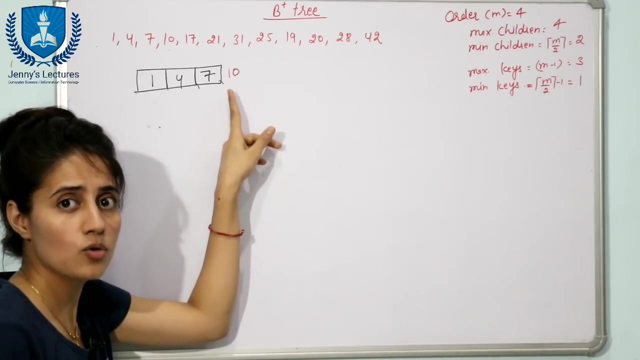 insert 7.. Next is 10.. Now where we can insert 10 after this? 7 here. But it is not possible. You cannot insert 10 in this node. Why so? Because it is overflow condition. Maximum keys in a node can be only 3 here. Fine in this case. So now, what should be done Now? 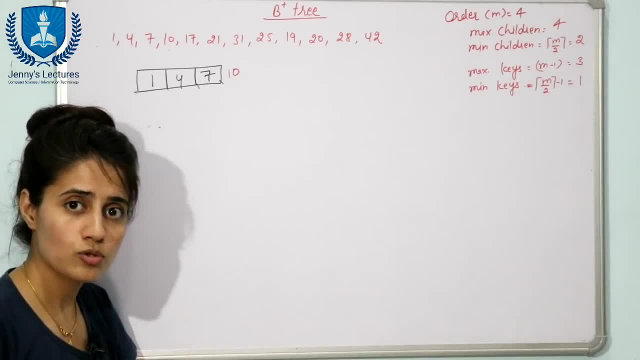 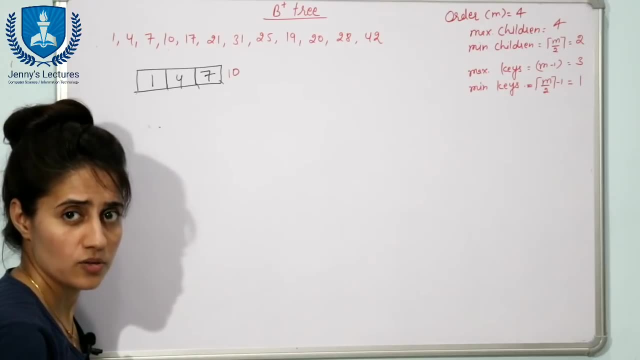 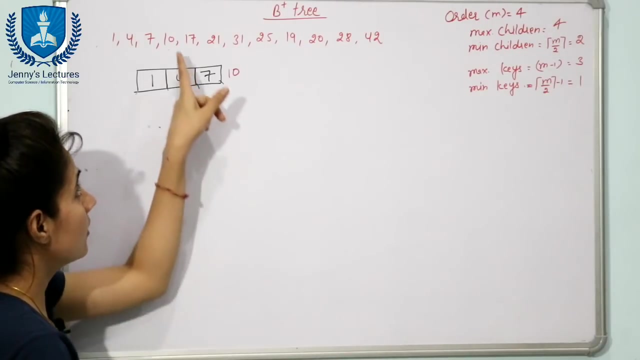 this node should be splitted Now. B tree and B plus tree also always grow towards root upward direction, not to the towards leaf direction, right, So we are going to find how, how this node is to be splitted. now Find out the middle element. Now, here we have 4 nodes, right, See, don't do this mistake that. 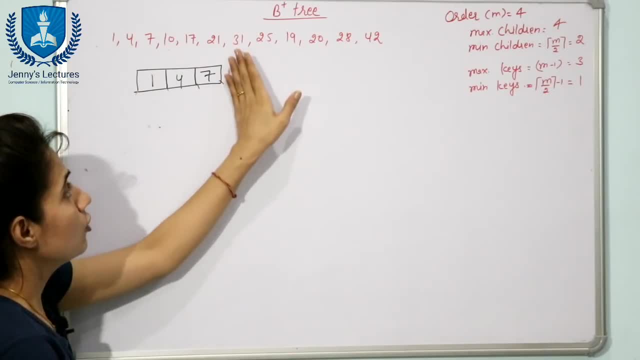 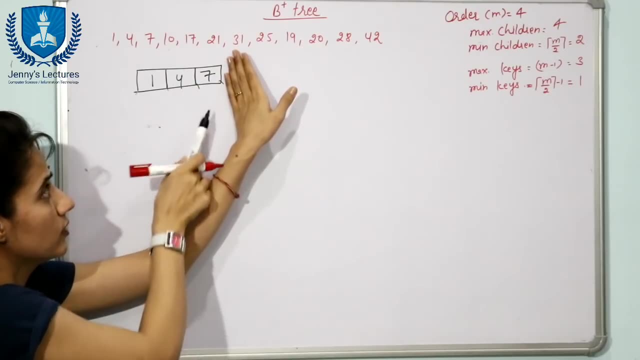 10 you are supposed to insert. We cannot insert 10 here, So remaining elements are 1, 2 and 3.. Find out the middle of this one: 4. 4 would go up and 1 is to the left of 4 and 7 is to the right of 4.. No, You are pretend. 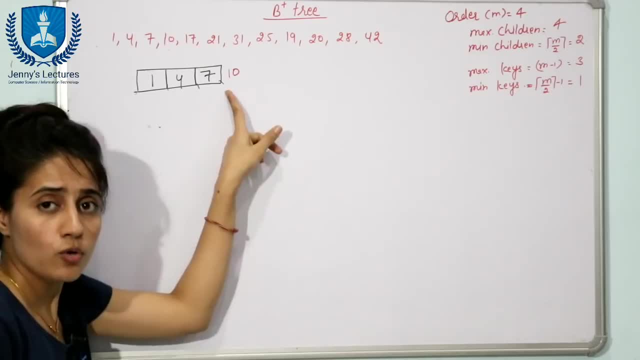 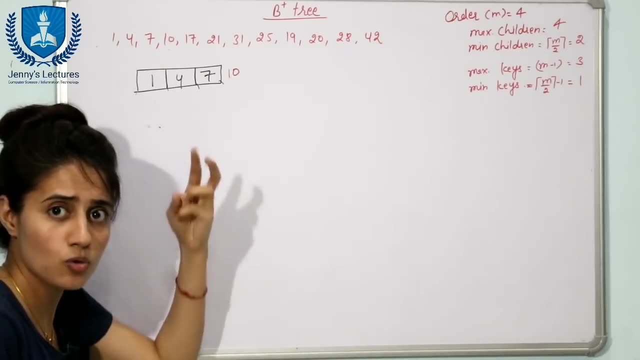 you have to pretend that, that you have inserted this 10 and now we are going to split this node, Right, But actually we haven't inserted because we cannot insert. Maximum limit is only 3 keys. So now the middle element can be this one and this one because we are having 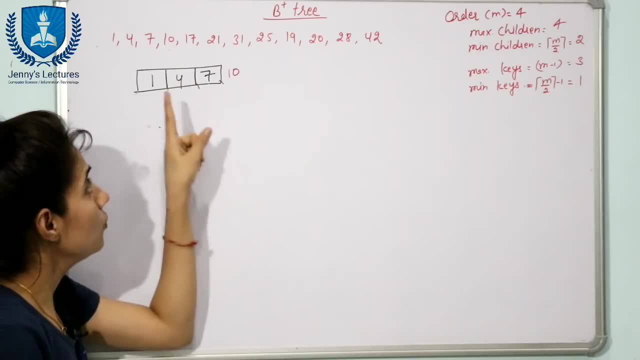 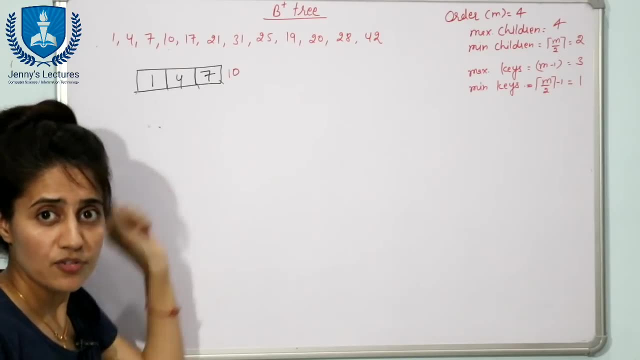 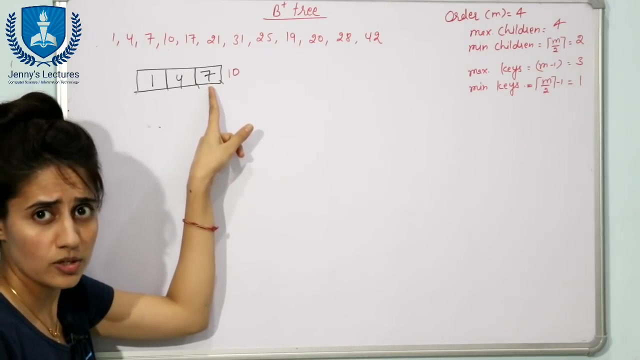 even factor 4.. Right, So if you, if you consider this as a middle element And you Split from this node, You will split from this data, Then the tree would be left biased. And if you consider 7 as a middle middle element and you split from this node, then you the. 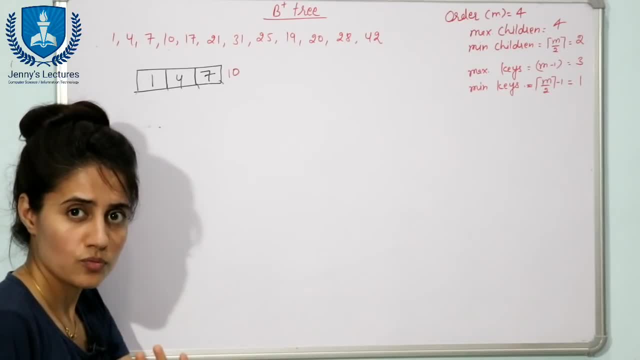 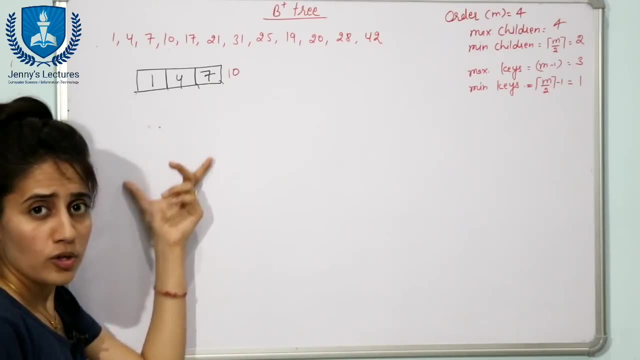 tree would be right biased. So it's up to you. You can take 4 also, you can take 7 also, But in starting, if you, if you construct the left biased tree, then during the completion of the complete tree you are supposed to follow that rule, also the left biased tree. And if 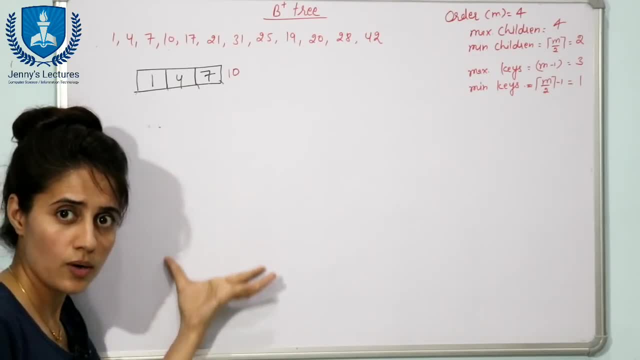 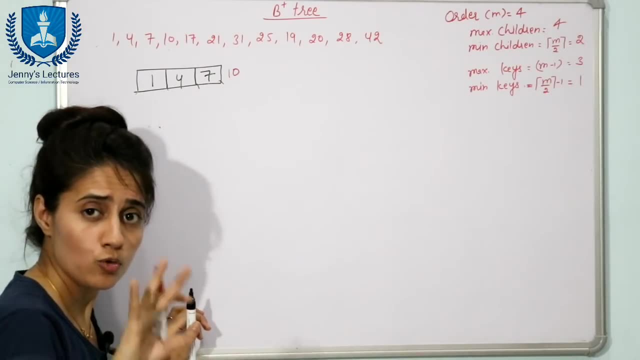 here you selected the tree as right biased. Then in the all the complete tree you are going to follow that rule, that right biased rule, Right. So here I'm taking 7 as middle element. I'm going to construct right biased tree Right. You can construct left biased also, and so your answer would be different. 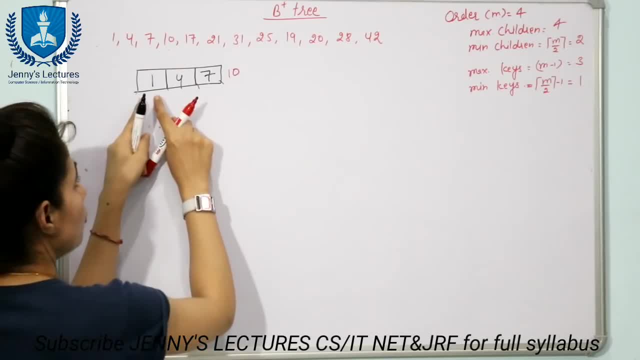 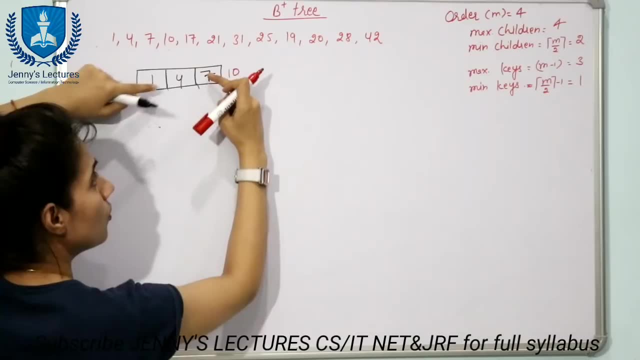 from my answer, But that is also correct, Right. So now 7. suppose 7 is middle element, So I'm going to split from this data. Now how splitting would be done. 7 would go one level up. or you can say to its parent: Now here we don't have any parent, So 7 would. 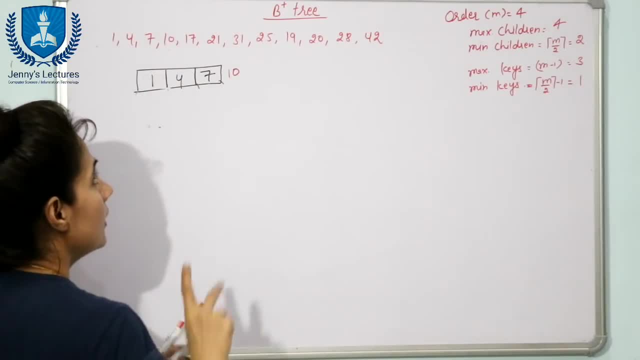 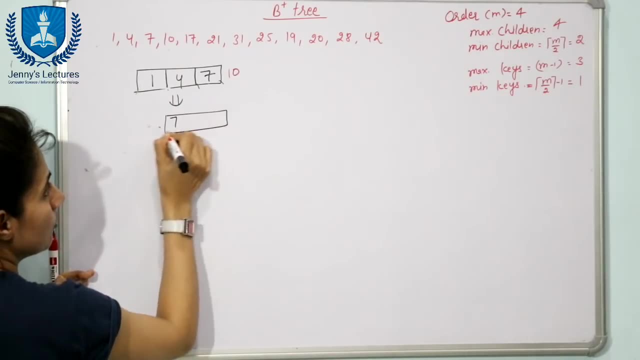 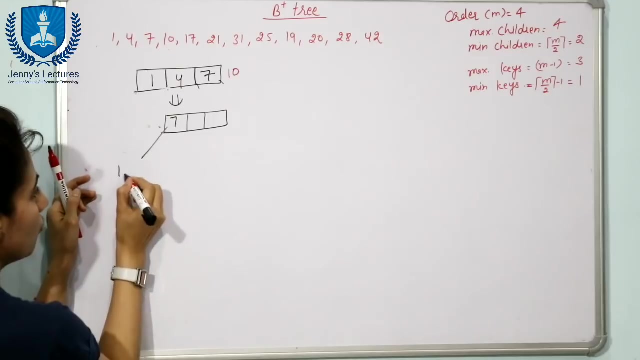 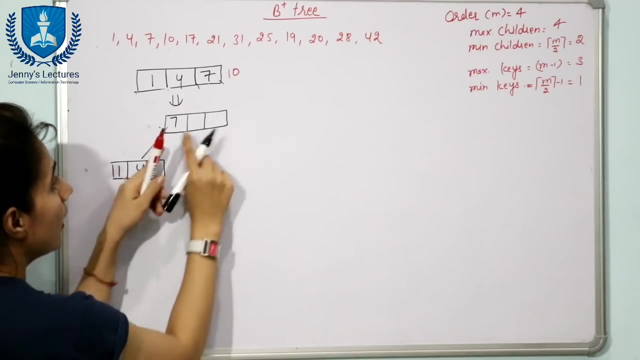 go up and that 7 would become parent. Now the tree would be something like this: See, 7 would go up, So create another node. The maximum capacity is 3 keys to the left of 7. to the left of 7, we have 1 and 4.. 1 and 4.. Right Here also, we can insert one more data. 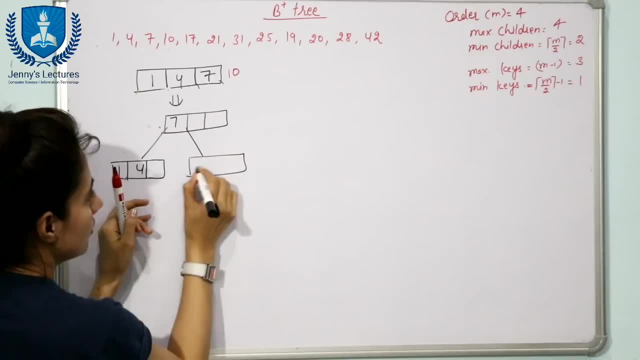 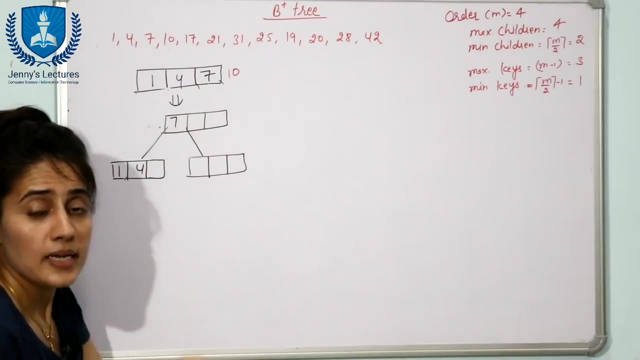 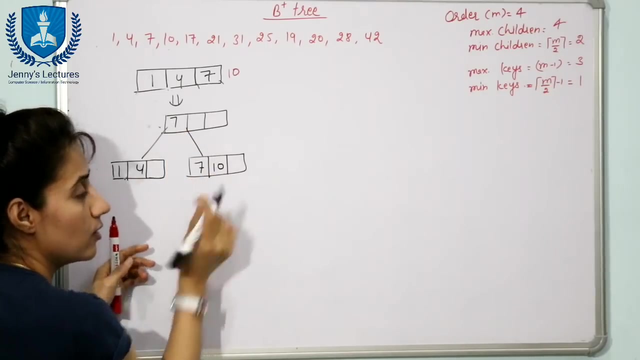 And to the right of 7. to the right of 7, what we can insert. Maximum capacity is 3 keys. To the right of 7, we have 10.. Right Plus, in B plus tree, what you will insert. You will insert this 7 also in this node, 7 and 10.. Why so? Because, see, I have told you in B plus, 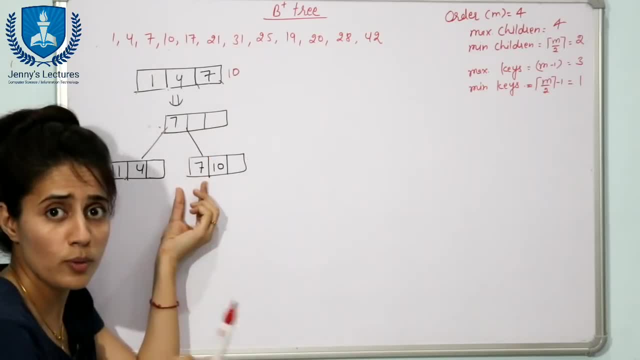 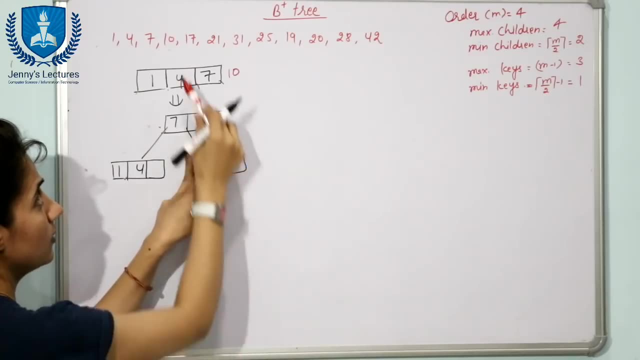 tree: the data, all the data. this data should be present in leaf node Right. So if you do not insert 7 here, So this is the leaf node and 7 is not present in the leaf node, So data should be present in leaf node. 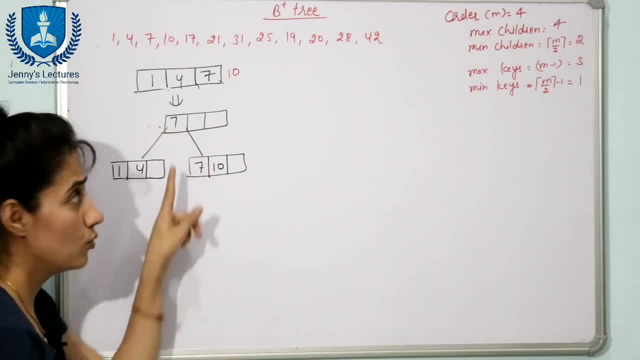 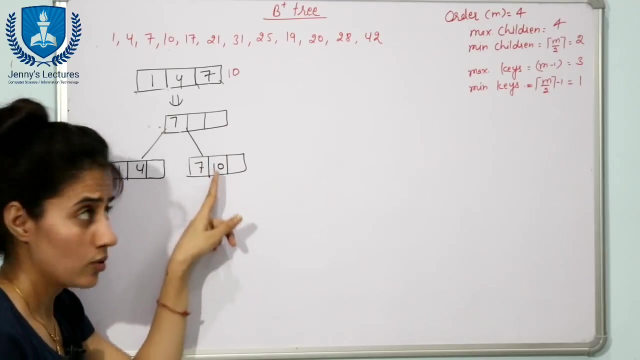 Now why you are inserting 7 to the right of this, this 7.. Why can't you insert 7 here? So another rule is that to the left of this one, all the data should be strictly less than this node Right, And to the right of this node, to the right of this node, from where? 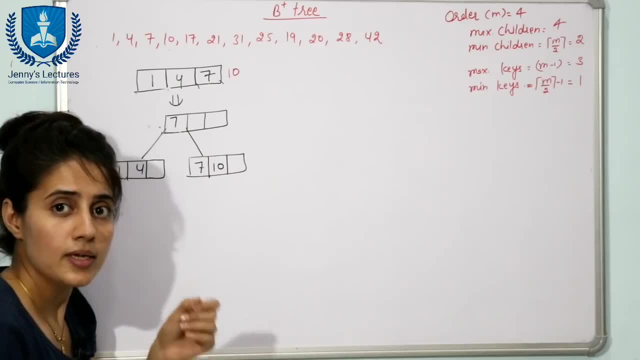 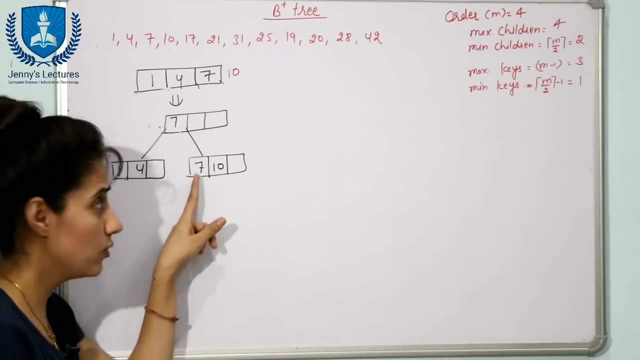 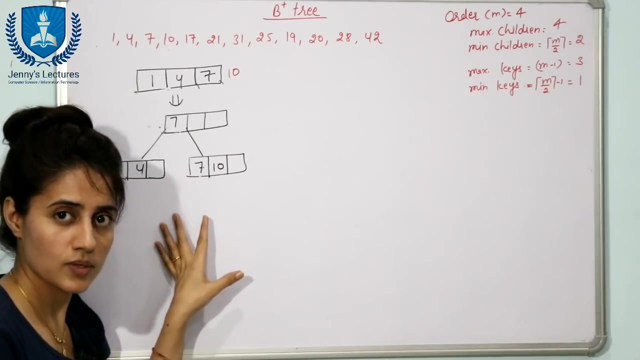 you are going to split to the right of that node. the data can be either greater than or equal to this node. So 7 is equal to this 7.. So we, we are going to insert 7.. 7 to the to this right side of this, 7 to the right side of the 7.. Right Now, see this: 7. 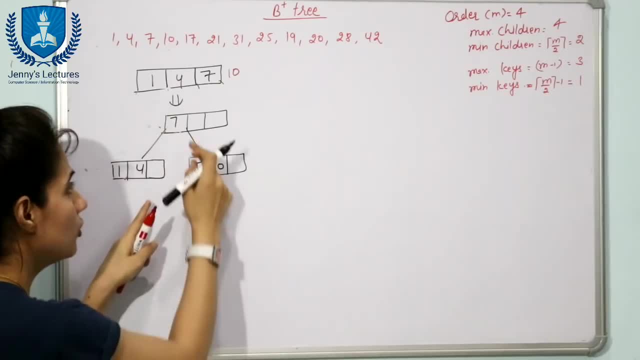 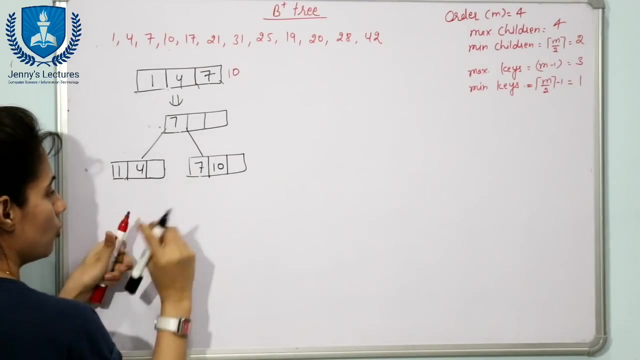 is only for the index value, or you can say, just pointer to this leaf node. Actual data is present here. Right Another thing I have told you: all the leaf node are connected with a link. The data is stored in the form of a link list. So this, this leaf node, is also. 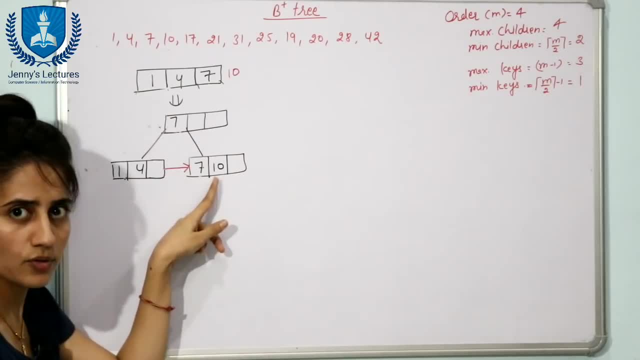 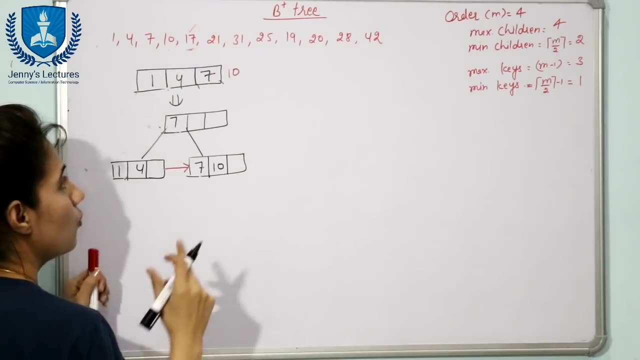 connected with this one using a link. Now, next, next, we are going to insert this: 17.. Now, where 17 can be inserted? Always, data is to be inserted in the leaf node that you have to take care. now, 17 is greater than 7.. 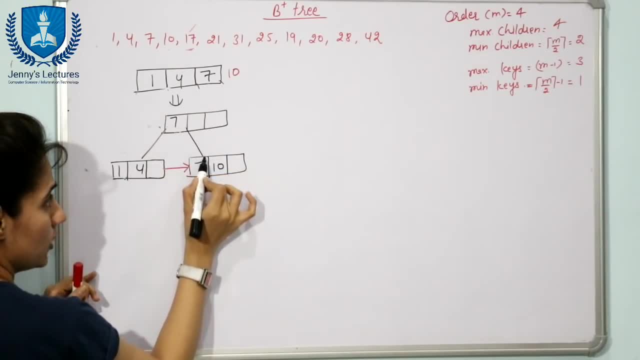 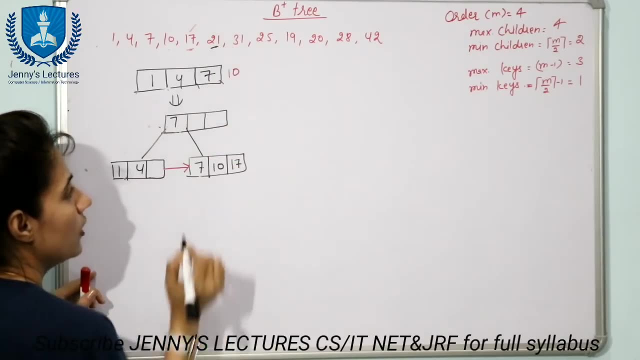 So go to go for this link: 17 greater than 7 greater than 7, this 10. so here you will insert 17.. Next is 21, where 21 can insert. 21 is greater than 7, greater than 7, 10 in. 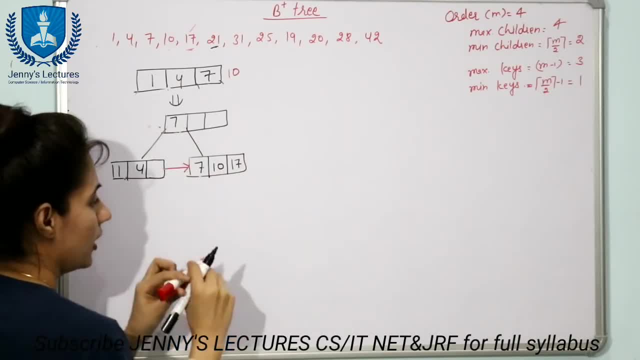 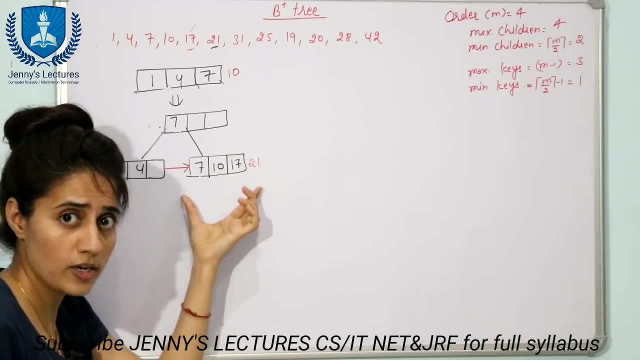 21.. Now remember, according to Yo eens, That this form is complicated. I can see 21, so here you can insert 21, but actually we cannot insert overflow condition, is there? now we have to split this node. now how splitting is to be done? the middle, i'll take the middle element. 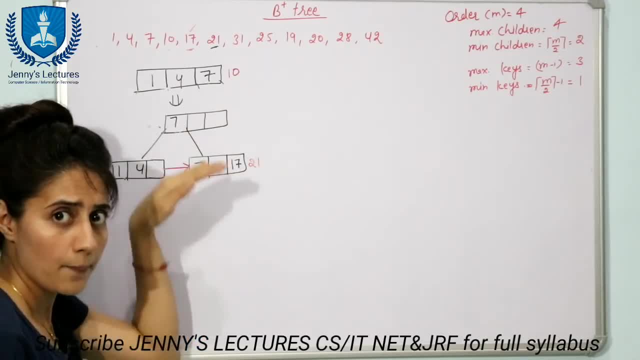 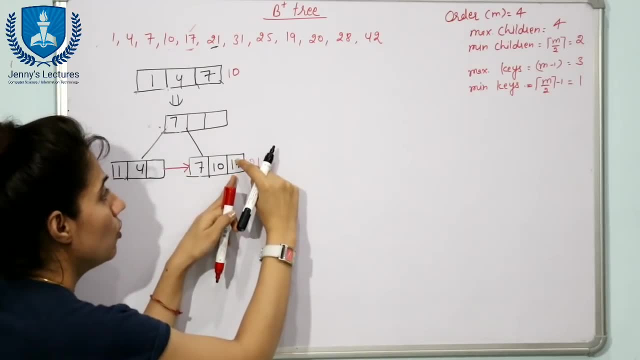 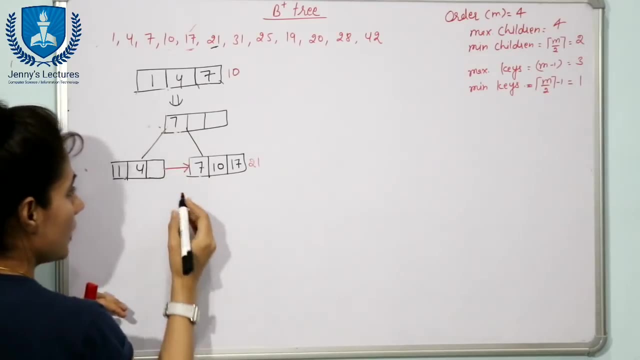 and that middle element would go one level up right. so now i'm constructing the right bias tree, so here i'm going to take 17 as middle element, so 17 would go to its parent node. or you can say one level up, so here you can insert 17, because two spaces are still free. so now the tree would 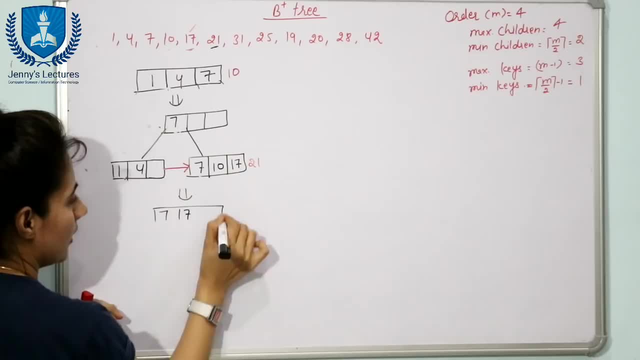 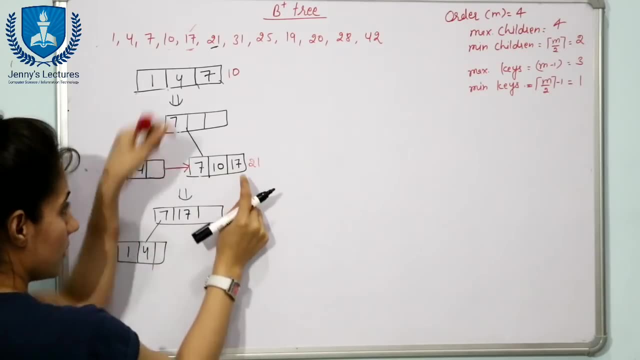 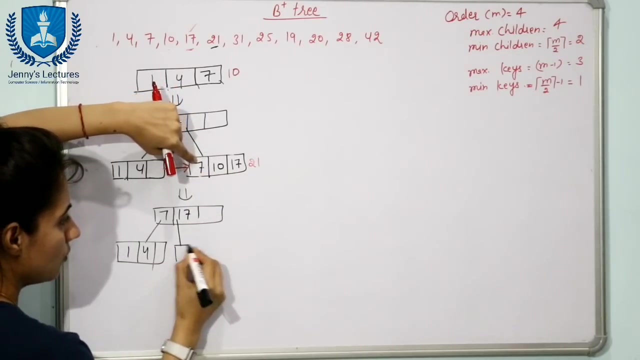 be 7 and 17, and here still we have one space left. same here we have 1 and 4 right and 17 would go up. so to the left of 17, 7 and 10. to the left of the 17, we have 7 and 10. right node is maximum. 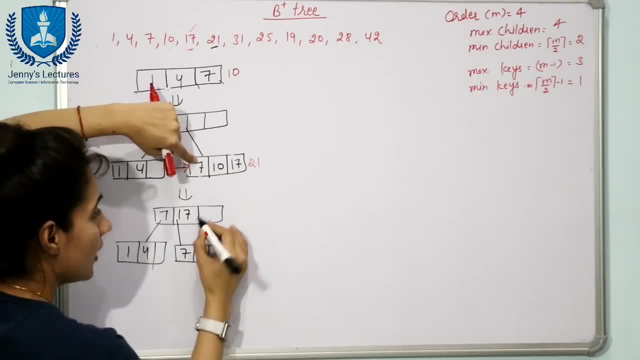 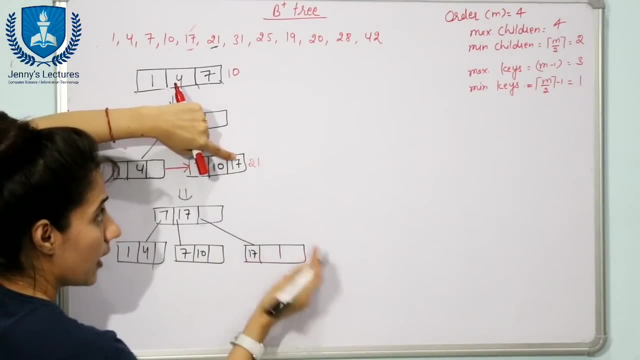 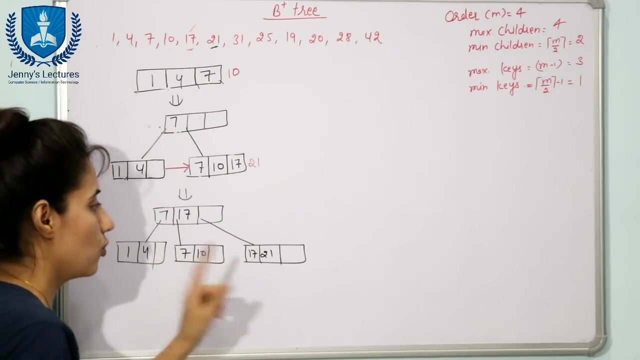 capacity of node is 3, so one space is free. and to the right of 17, to the right of 17, 17, 17, 17. the data would be 17 and 21. right, because the data should be present in leaf node. fine, so now. next is 31. now where you can insert 31 greater than 7, greater than 17, so go to this link. 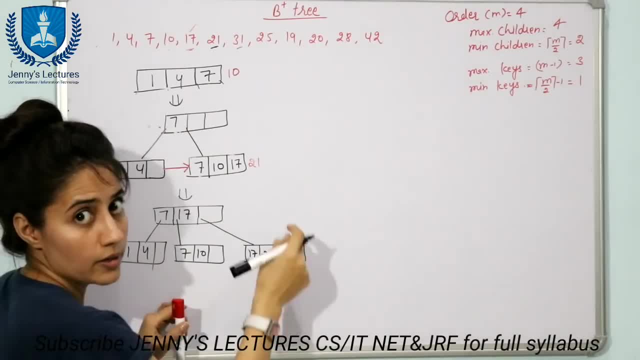 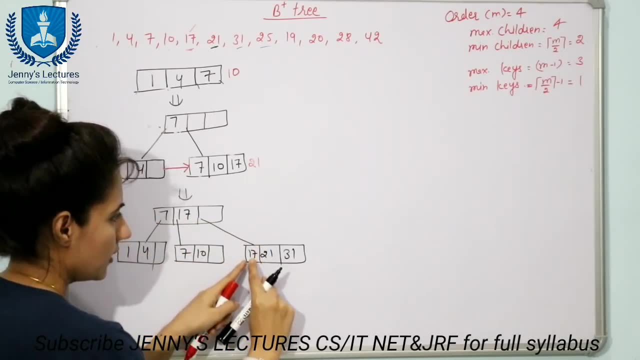 greater than 21, so we will insert 31 here only now. next is 25, where you can insert 25. 25 has greater than 7, greater than 17, so go to this link: greater than 17, greater than 21 and less than 31. so 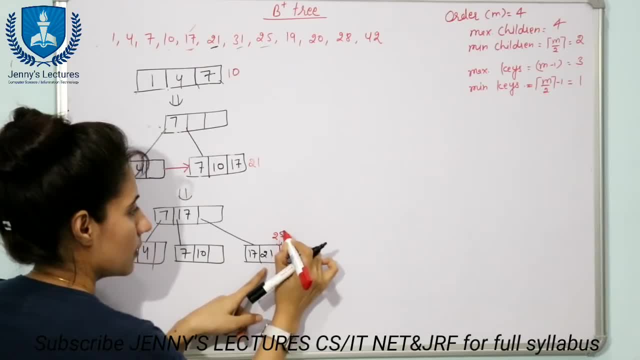 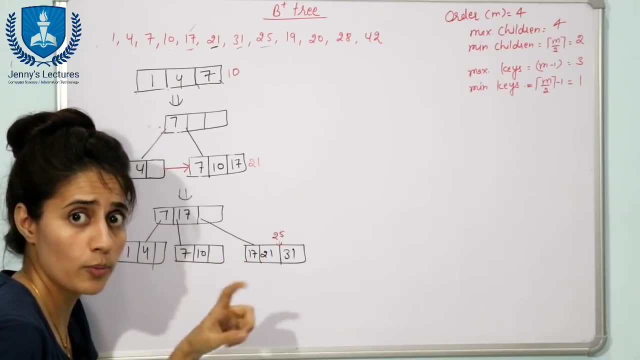 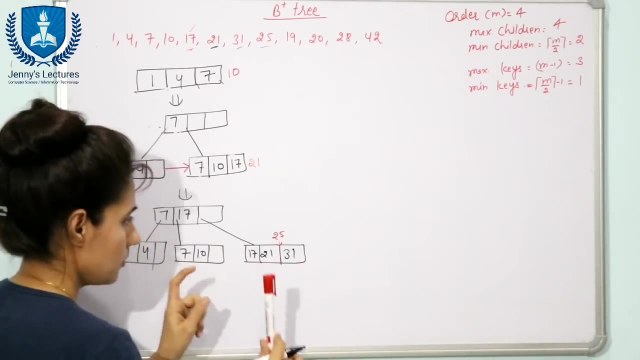 so where you can insert 25 here after 21, before 31, right, because, uh, it is a bst also, you have to follow the property of bst. fine, now this cannot be done. overflow condition is there. now splitting would be done. now, splitting is what find the middle elements sounds. i am going to construct the right bias. 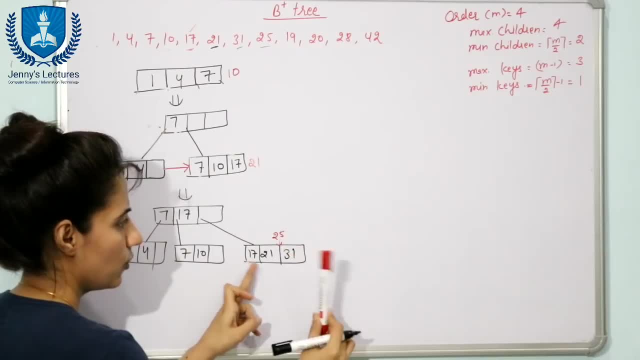 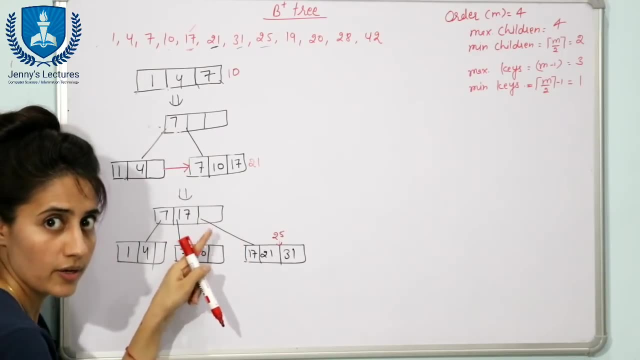 tree. so middle element out from this: 17, 21, 25 and 31 is 25. so 25 would go one level up. so 25 would would go here, only fine. now i am going to update this, this tree only. so 25 would go here. so still. 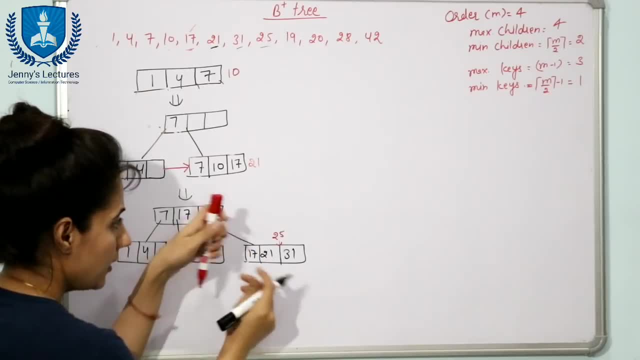 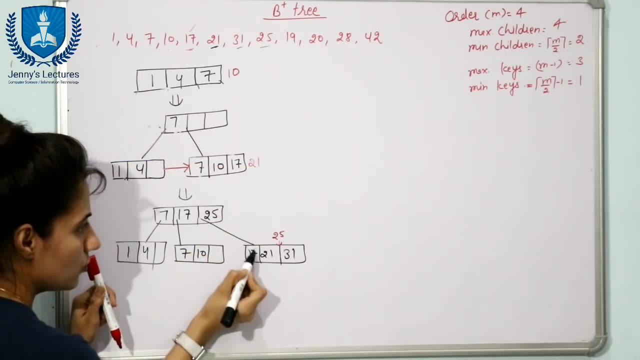 we have one space left so we can insert 25 here. and if you are splitting from this northern to the left of 25, we have 17 and 21. fine, to the left of this, we have 17 and 21 and to the right of 25. 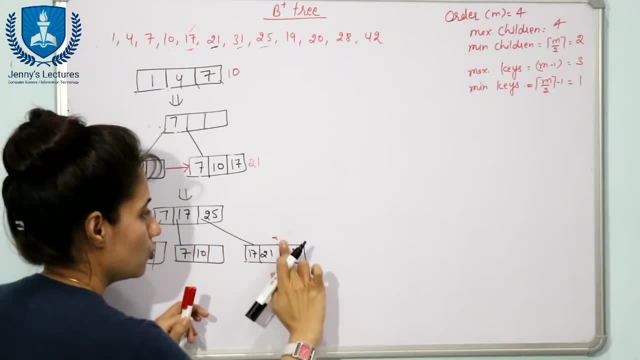 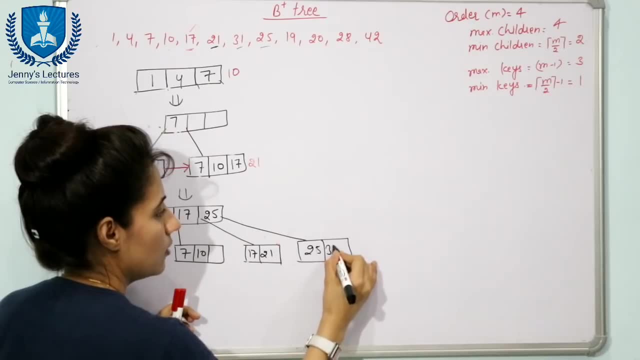 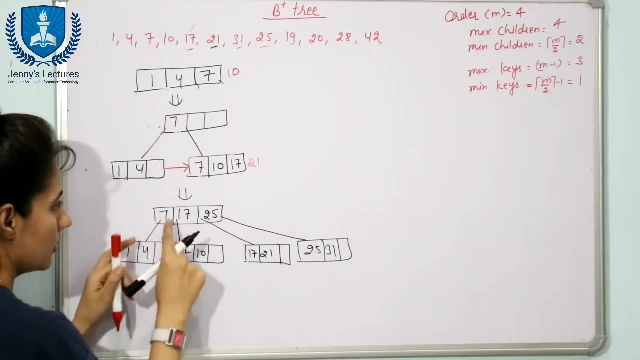 what would have 25 and 31. so, to the right of 25, you will have 25 and 31, and one node is still free, and here also, one node is still free. now, next is 19, where you can insert 19. 19 is greater than. 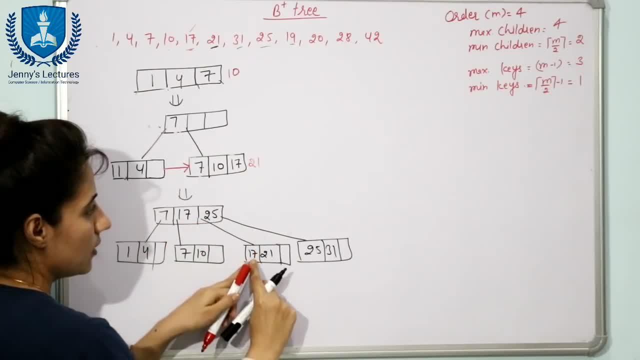 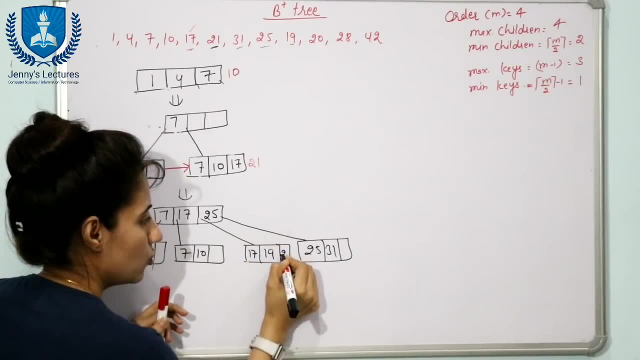 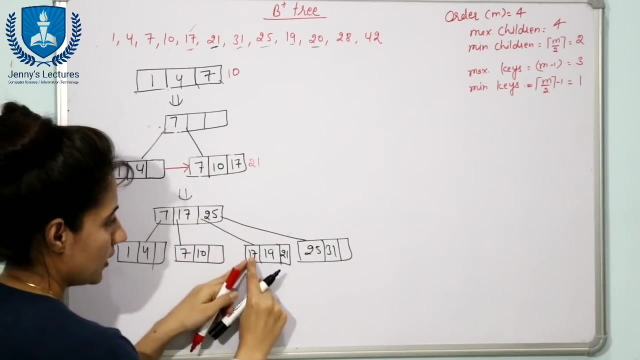 17 but less than 25. so go to this link: 19 greater than 17, but less than 21, less than 21. so here you will insert 19 and 21 would go here. next is 20, where you can insert 20 greater than 17 less than 25. greater than 17 greater than 20. 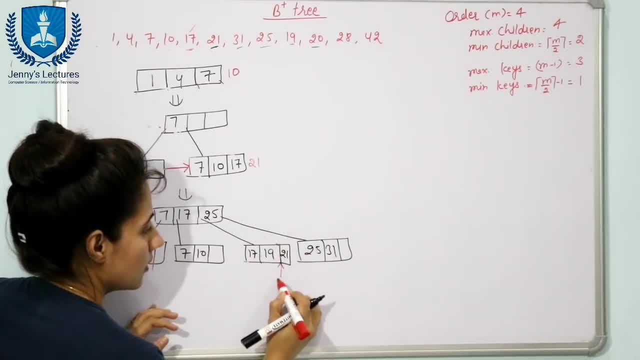 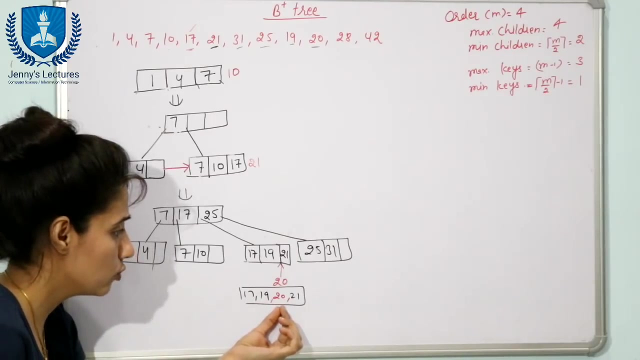 and less than 21. so you can insert 20 at this place, 17. here you will write 17, 19, 20 and 21. right, this node will be something like this. but you cannot insert 21 here. you have to split this node from where you are going to split. middle element is 20, so 20 would. 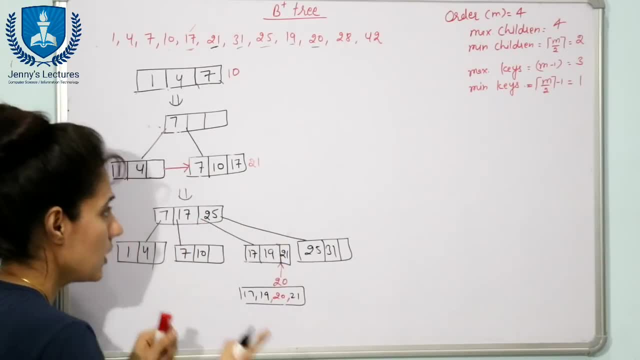 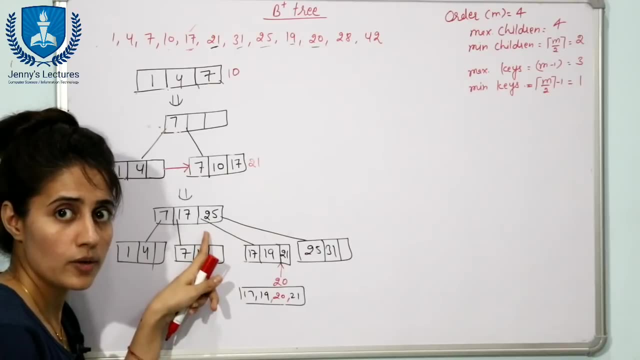 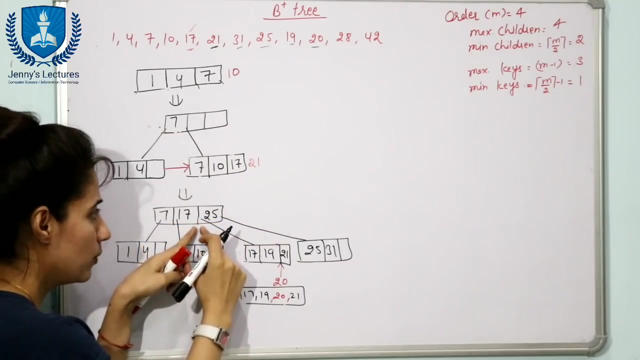 go up, so fine, and here also now you cannot insert 20 because this node is also full. now you will repeat the same step of splitting. you will split this node also, fine, and that that node, that from where you are going to split that element, would go one level up, fine. so i am going to, first of 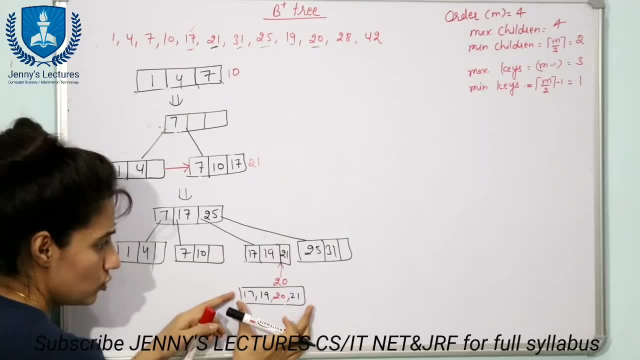 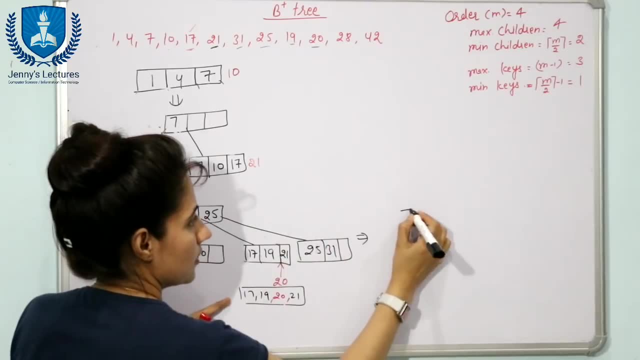 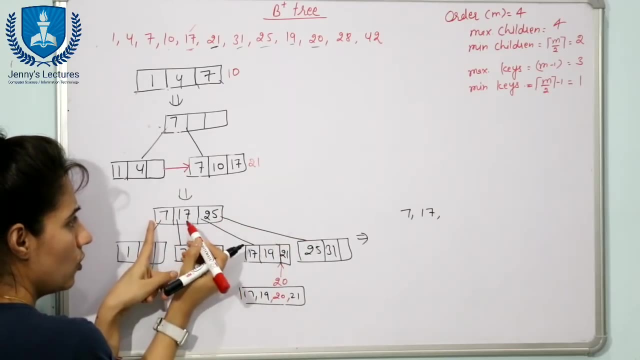 all do one splitting from this node only fine. so if this node is splitted, then 20 would go one level up. so now, now this tree would be something like this: 7, 17. so now, if 20 would go one level up, so in this node where 20 can go after this 17, here you will write 20 and here you will write 25. 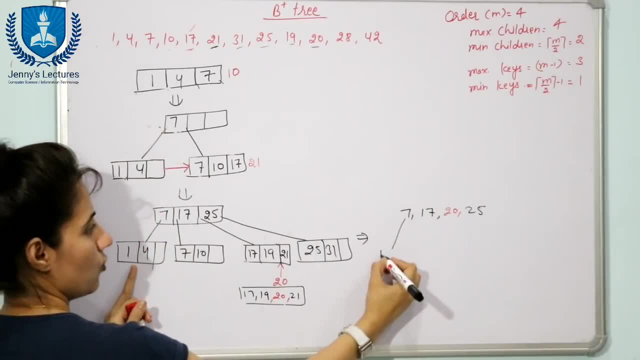 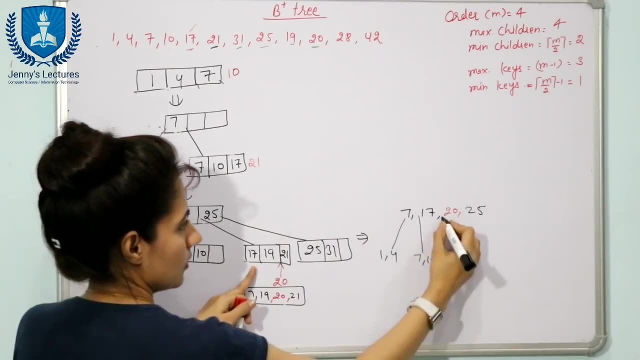 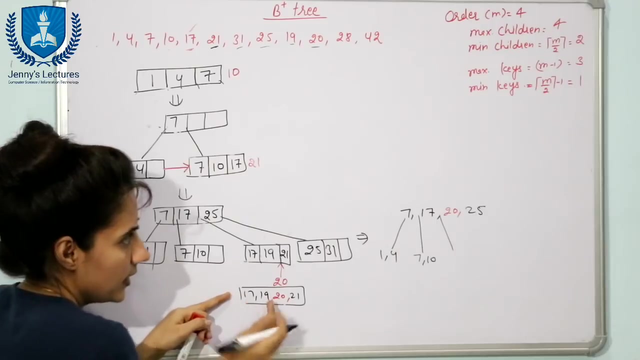 right and to the left of 7, we have 1 and 4. to the left of 17 we have 7 and 10 to the right of 17. now, from here, splitting is done, 20 would go up. so to the left of 20, we have 17 and 19. to the left of. 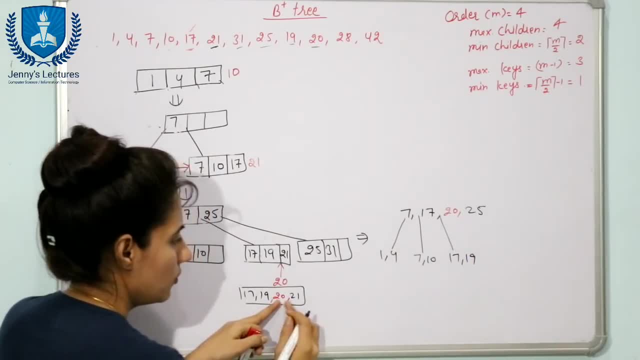 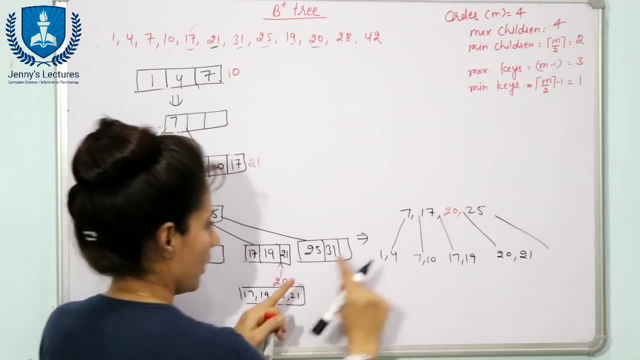 20 we have 17 and 19, and to the right of 20 we will have 20 and 21. so here you will have 20 and 21, and to the right of 25 you will have 25 and 31. but this is the intermediate stage. we are not done. 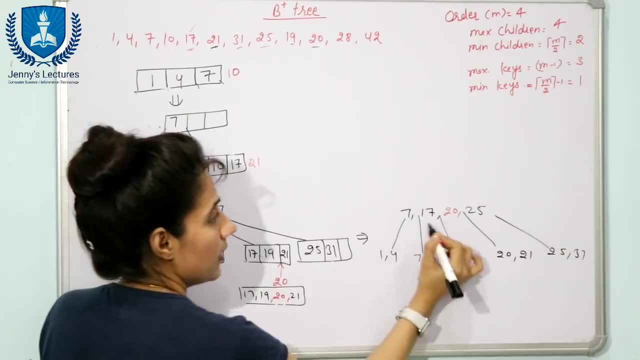 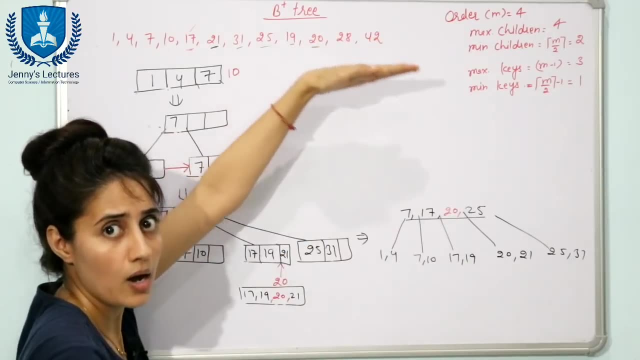 that is why i am drawing this, something like this now again. this is not all. this is not possible. you have to split this node also now from here. middle element is 20, 20 would go one level up. so after that, after that, after this, splitting tree would be something like this: 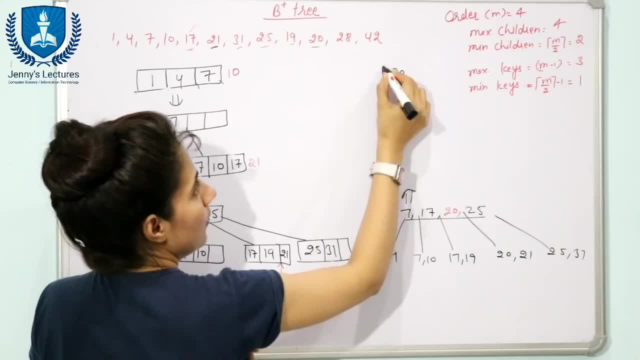 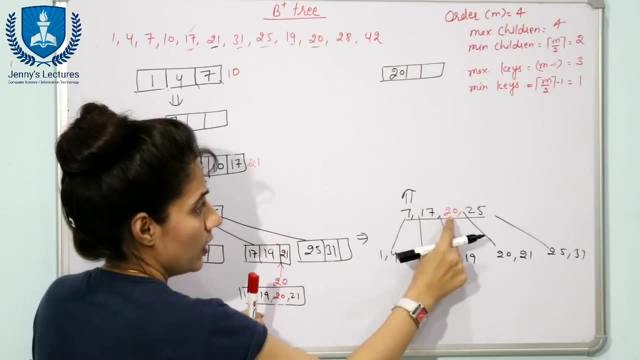 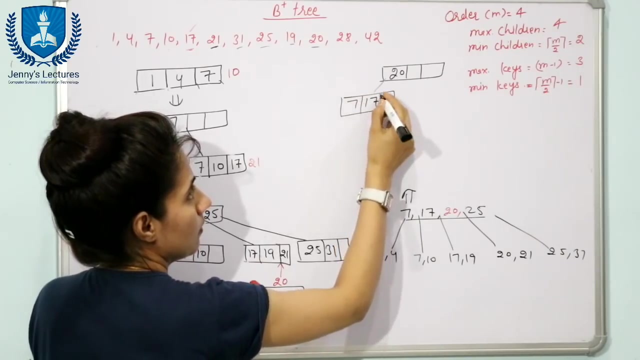 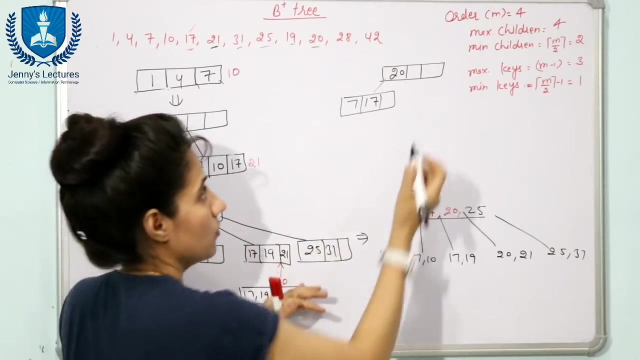 see, 20 would go one level up when another node would be created, having maximum space of three keys. to the left of 20, we have 7 and 17, 7 and 17. at this level, right to the right of 20, according to the rule, what should be the keys 20 and 25. so, to the right of 20, we should have 20. 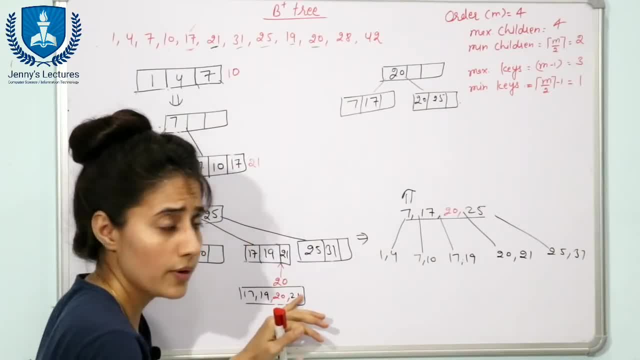 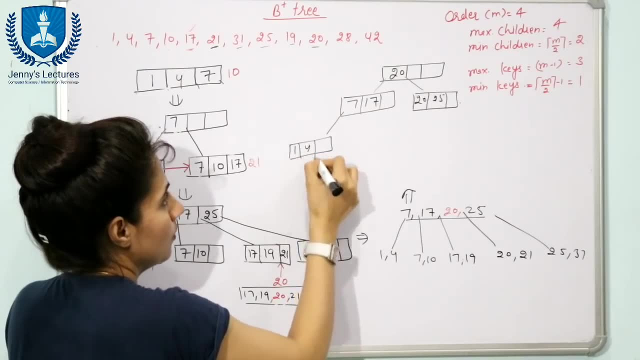 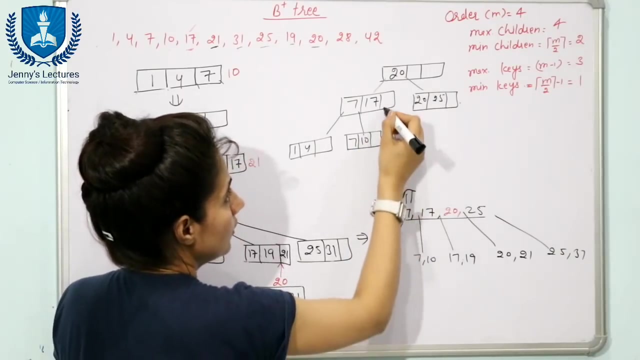 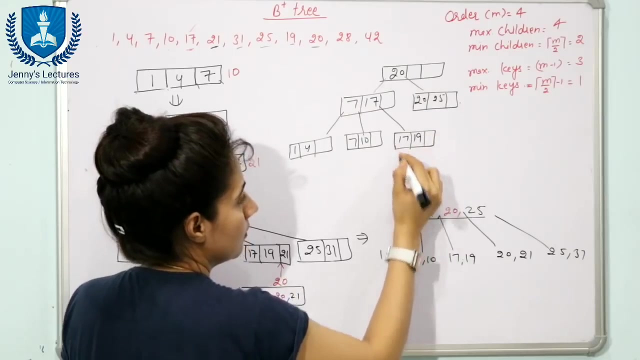 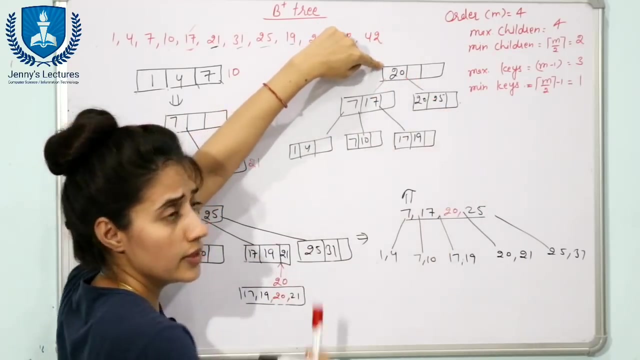 and 25 right, and, as it is, these elements would be one and four to the right of this, we have 7 and 10 to the right of 17, we have 17, 19 right now. these are leaf nodes, right, and this is internal node, and this is also internal node. 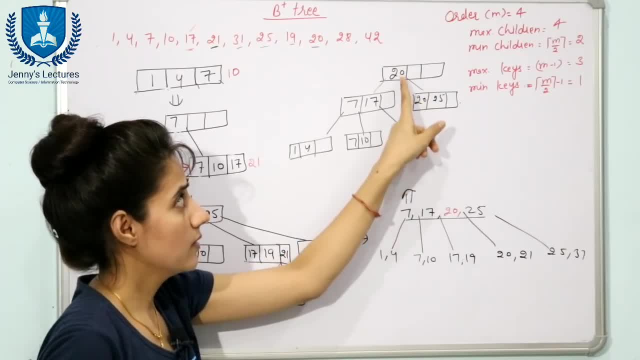 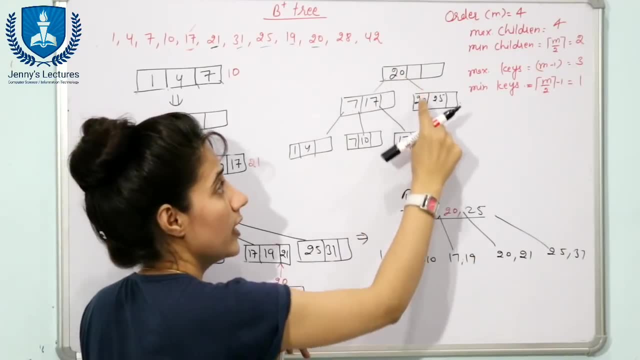 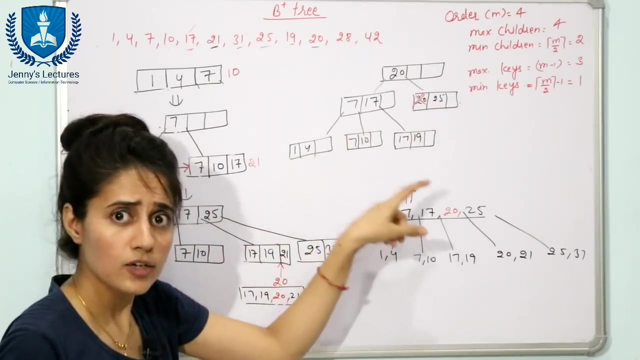 so now the rule is these keys. this cannot be repeated in internal nodes. so here you have written just 20. so here you cannot write this 20, you are going to cross 20 from here, because what actual data is in leaf node and in internal nodes we just have indexes. so what is the point to 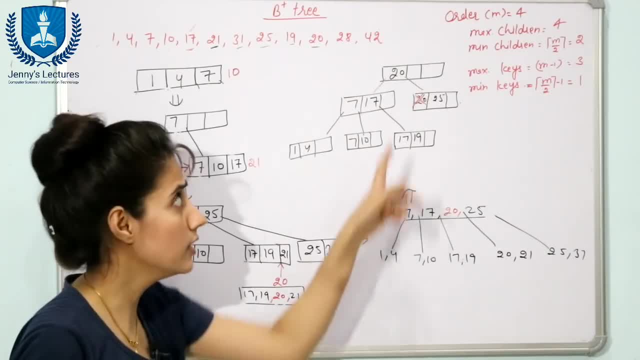 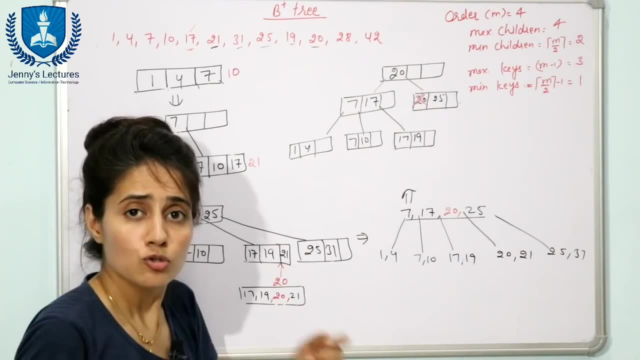 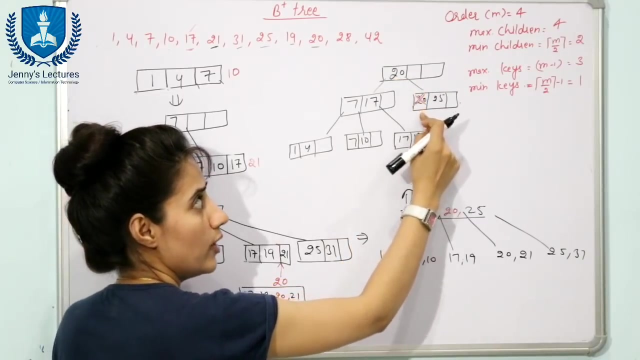 repeat the same index again and again. we just need one index and using that index or using that pointer only we can reach to the actual data, right? so that is why in this internal nodes we are not going to repeat the same data. so here we have written 20, so we are not going to write 20 here. 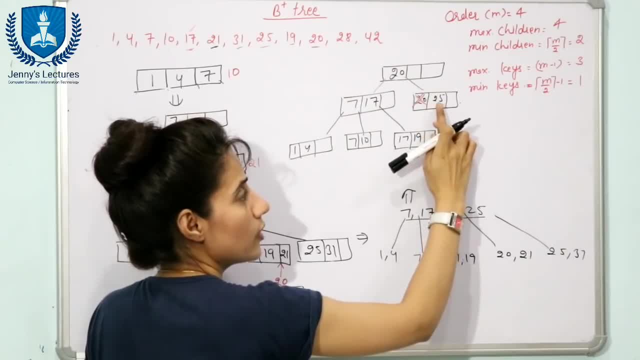 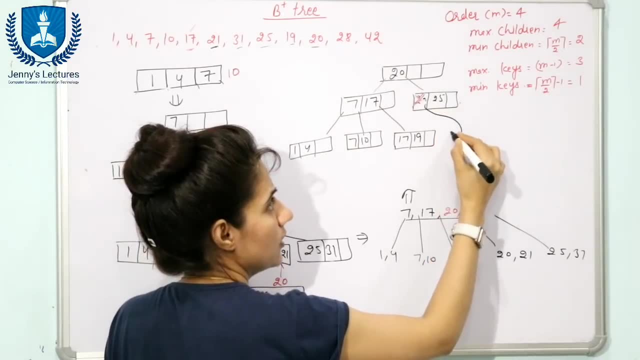 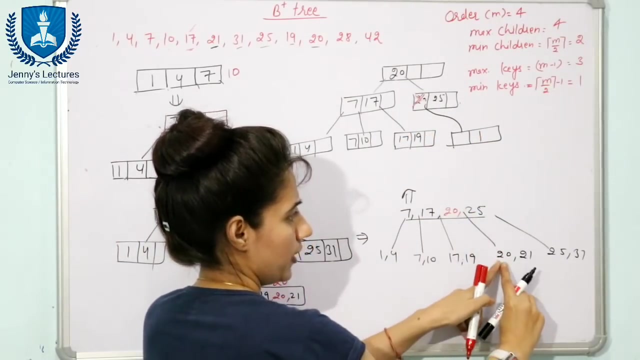 fine, so here you will. you will just just write 25. so now here, 20 is not there. to the left of to the left of this 25, the data is to the left of 25. the data is what 20 and 21 see to. to the left of 25, we have 20 and 21. 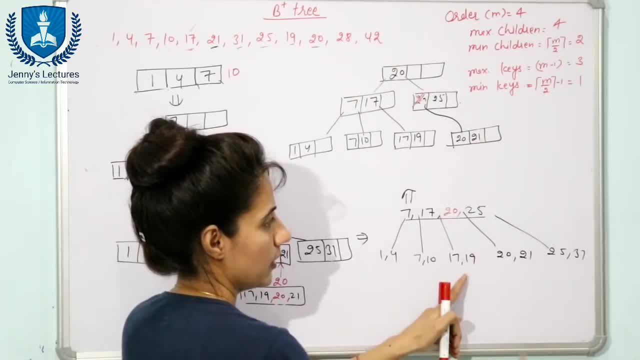 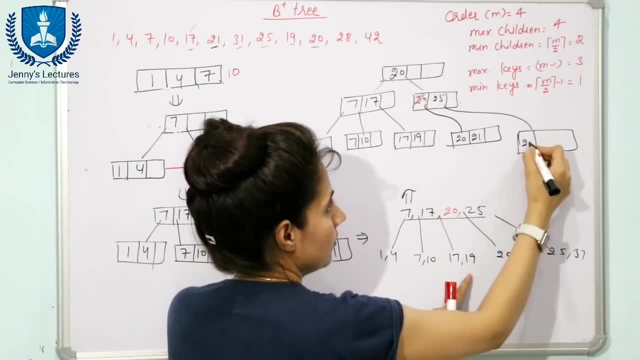 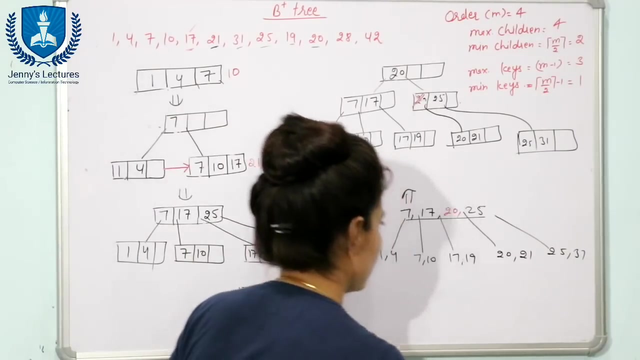 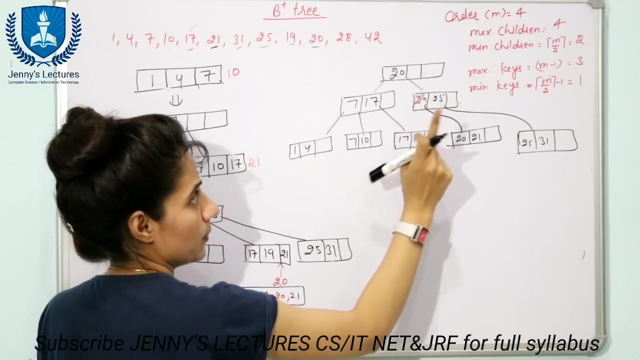 20 and 21, fine, and to the right of 25 we have 25, 25, 25 and 31, so this is from this stage. the tree would be something like this, so i'm going to rub this intermediate stage. fine. now here 20 is not present, so here we don't have any. element 20 is not there. 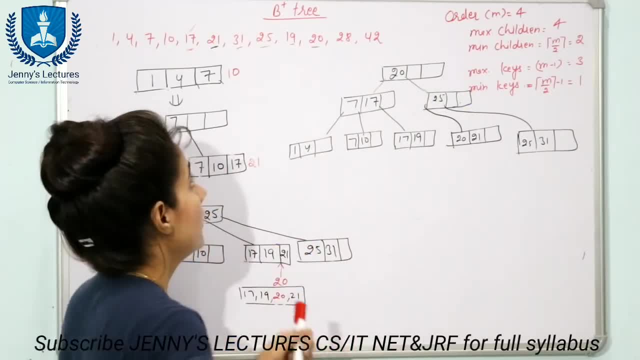 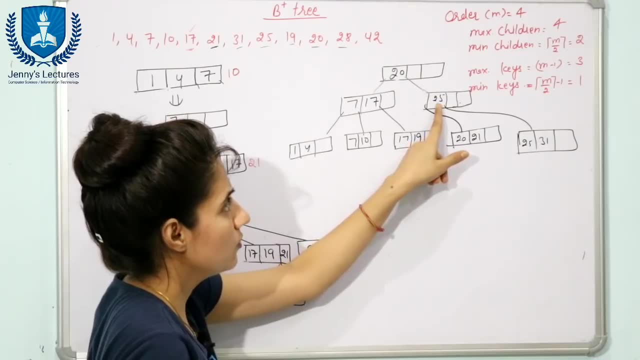 fine, you just have 25 now. next next is 28. now where 28 can go, 28 is greater than 20, yes, greater than 25. go to the right side of the tree. so here 20 is not present, so here we don't have any element. 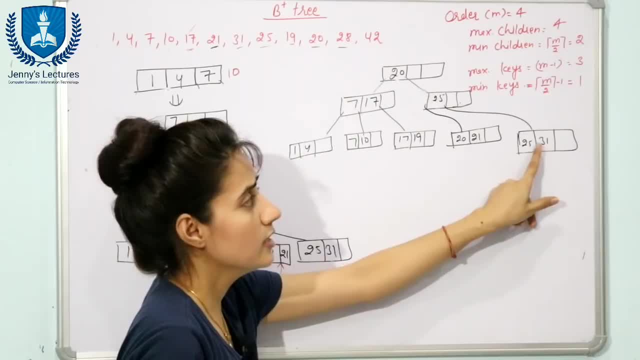 20 is not present, so here we don't have any element. 20 is not present, so here we don't have any element. of 25. go to this link: greater than 25, but less than of 25. go to this link: greater than 25, but less than. 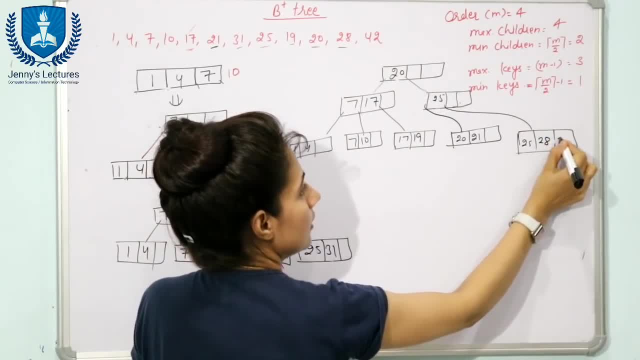 of 25. go to this link. greater than 25, but less than 31. so here you will insert 28, here you will write 31. so here you will insert 28. here you will write 31, so here you will insert 28, here you will write 31. next is 42. 42 can go to right of 30. 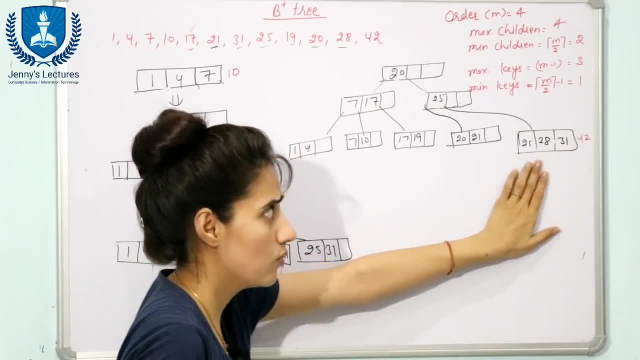 31, next is 42. 42 can go to right of 30. 31, next is 42. 42 can go to right of 30: one. so here you can insert 42, but actually one. so here you can insert 42, but actually one. so here you can insert 42, but actually you cannot insert. this is overflow. 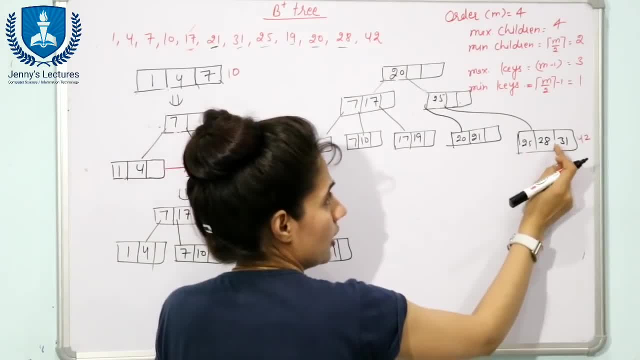 you cannot insert: this is overflow. you cannot insert. this is overflow. condition again: splitting would be done. condition again: splitting would be done. condition again: splitting would be done and middle element is 31: 31 would go one and middle element is 31: 31 would go one. 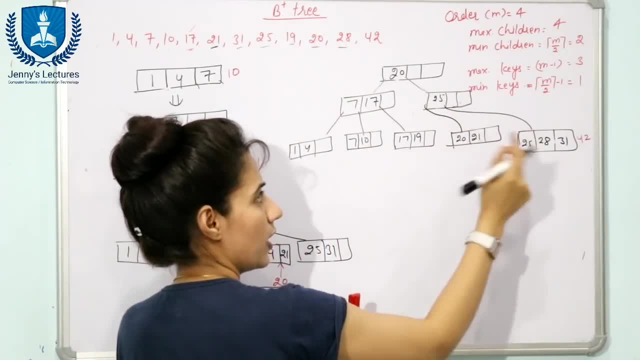 and middle element is 31. 31 would go one level up here. only we have a two space level up here. only we have a two space level up here. only we have a two space left. so that is fine, 31 can go here left. so that is fine, 31 can go here. 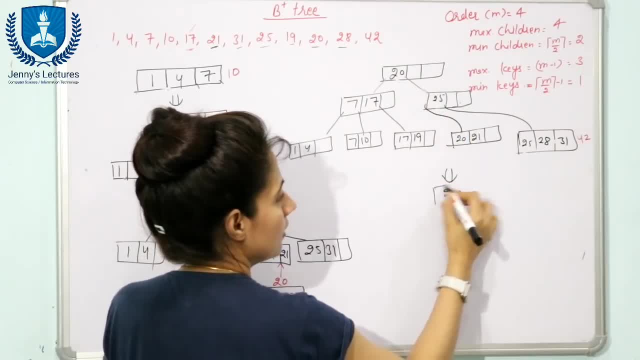 left. so that is fine. 31 can go here. so after this, the tree would be something. so after this, the tree would be something. so after this, the tree would be something like this: we have 20 like this. we have 20 like this. we have 20 here. we have 7 and 17. 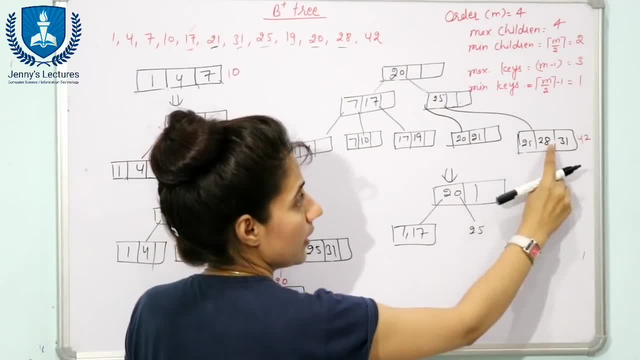 here we have 7 and 17, here we have 7 and 17. to the right of 20, we have 25, and to the right of 20, we have 25, and to the right of 20, we have 25, and and 31, 31 would go one level. 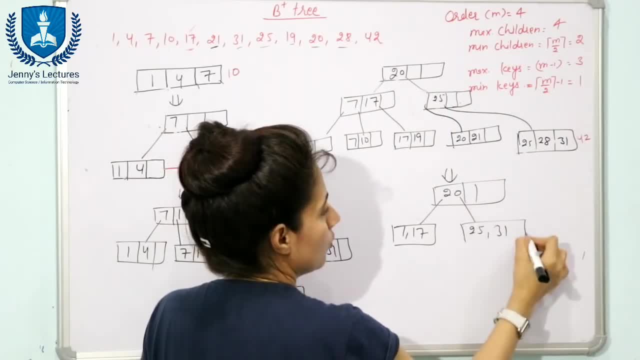 and 31, 31 would go one level and 31, 31 would go one level up. so here here we have 30 up. so here, here we have 30 up. so here here we have 30, one, one, one, right, right, right, these elements would be same: one and four. 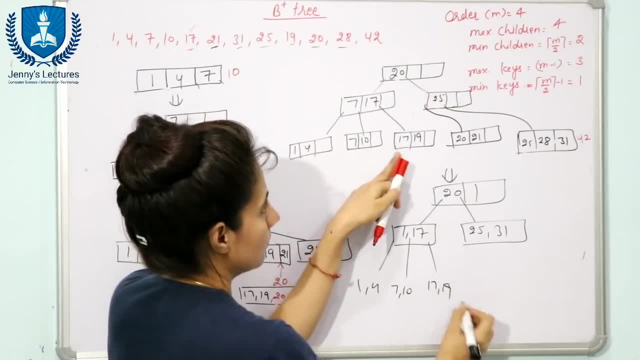 these elements would be same: one and four. these elements would be same: one and four. here you will write 7 and 10. here you will. here you will write 7 and 10, here you will. here you will write 7 and 10. here you will write 17 and 19. fine. 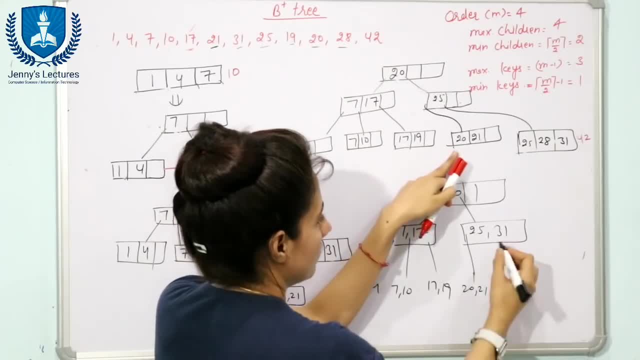 write 17 and 19 fine. write 17 and 19 fine. to the left of 25 would be 20 and 21 to the left of 25 would be 20 and 21 to the left of 25 would be 20 and 21. right and now. 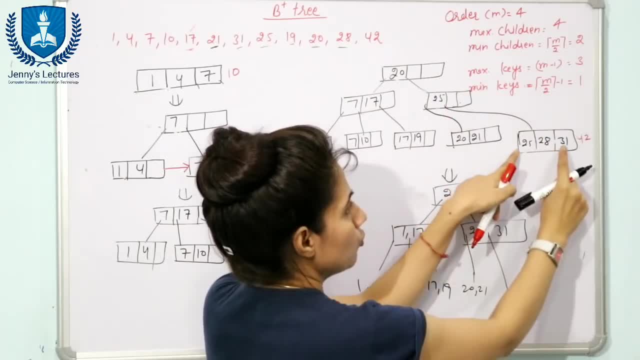 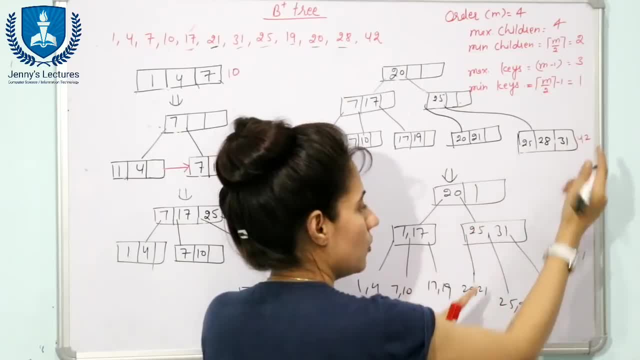 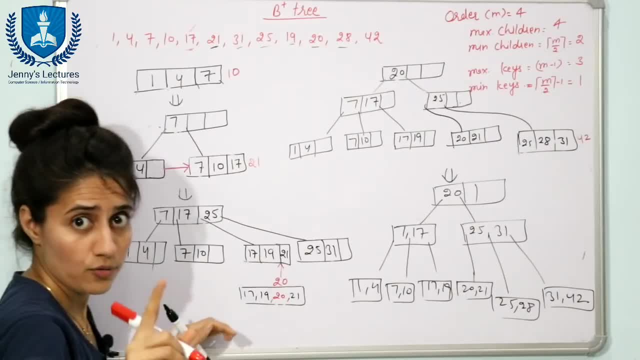 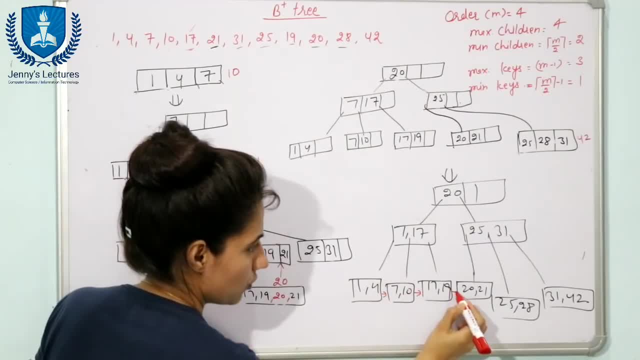 this link will all the present, in all the between all the leaf nodes from this, between all the leaf nodes from this, between all the leaf nodes from this leaf node to this one, from this to this leaf node to this one, from this to this, from this to this, from this to this from. 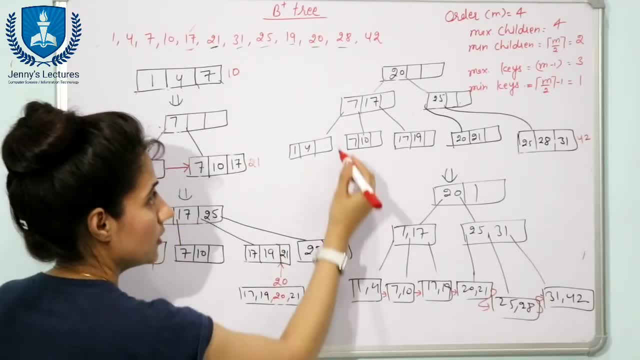 from this to this, from this to this, from from this to this, from this to this, from this to this to this, to this, this, this, so this link would be present in all the. so this link would be present in all the. so this link would be present in all the leaf nodes, like this: 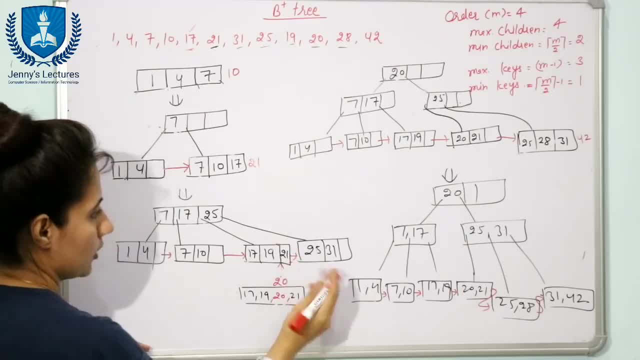 leaf nodes like this, leaf nodes like this. you have to insert this link also. you have to insert this link also. you have to insert this link also. and from here to here something like, and from here to here something like, and from here to here something like this: 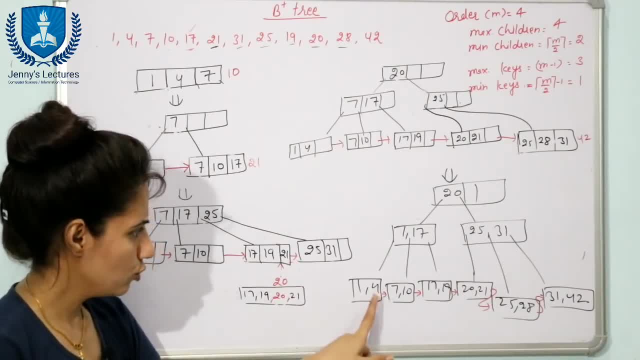 this, this right, right, right. this is the final b plus tree here also. this is the final b plus tree here also. this is the final b plus tree here also. you are having, uh, the space of the node. you are having, uh, the space of the node. you are having, uh, the space of the node is having space of three keys. so here i. 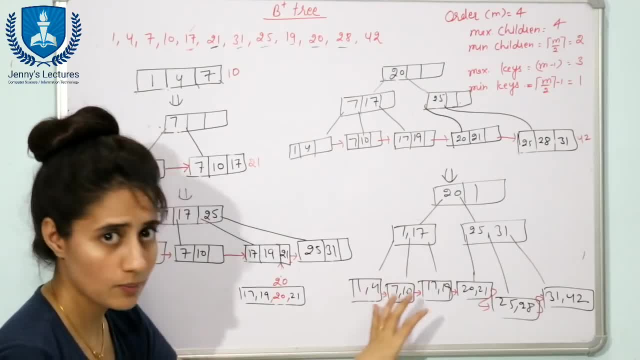 is having space of three keys, so here i is having space of three keys, so here i have shortage of space. that is why i have shortage of space. that is why i have shortage of space. that is why i have just have, just have just made a little bit mashed up, fine. so i 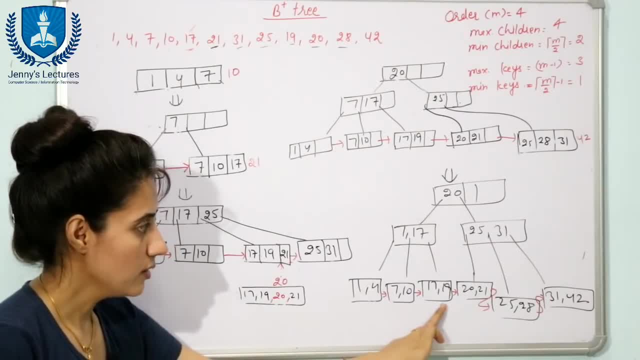 made a little bit mashed up, fine. so i made a little bit mashed up, fine. so i hope you are getting this is the tree, hope you are getting this is the tree. hope you are getting this is the tree. fine, these nodes are having space of. fine, these nodes are having space of. 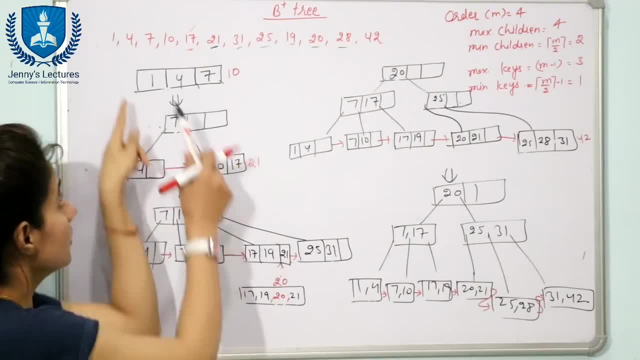 fine. these nodes are having space of three keys. right maximum, you can insert three keys. right maximum. you can insert three keys right maximum. you can insert three keys. now see as you can see this. three keys now see as you can see this. three keys now see as you can see this. this data, this data is present in the 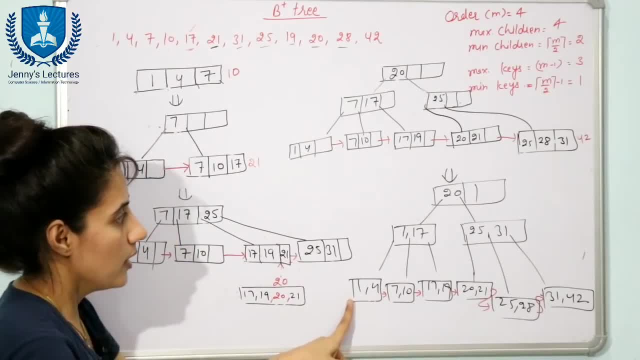 this data, this data, this data is present in the. this data, this data, this data is present in the leaf node. all the data you can leaf node all the data you can leaf node all the data you can check fine, and in this internal nodes: check fine. and in this internal loads. 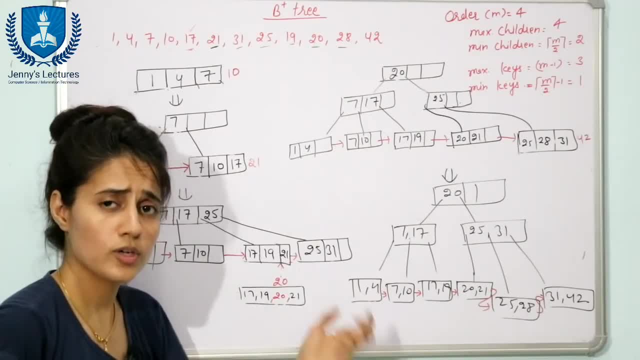 check, fine, and in this internal loads, we are having just the indexes, we are having just the indexes, we are having just the indexes, fine, or you can say pointers- fine, or you can say pointers- fine, or you can say pointers as well as these, these leaf nodes are. 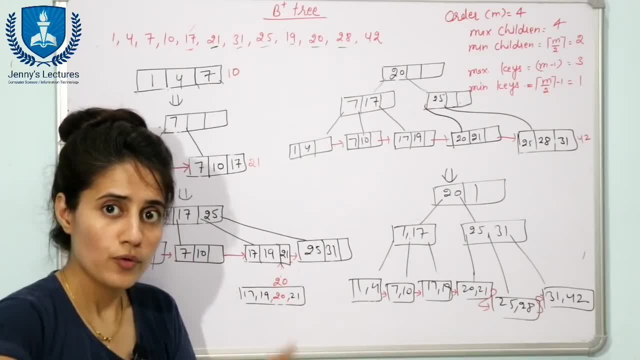 as well as these. these leaf nodes are as well as these. these leaf nodes are also linked with each other, also linked with each other, also linked with each other. so, when you are going to access a data, so when you are going to access a data, so when you are going to access a data, that is why, see, that is why in b plus 3. 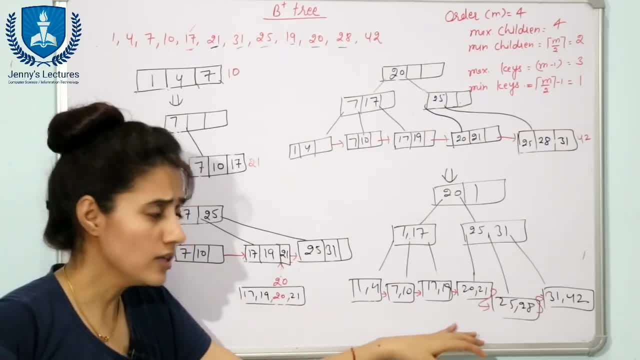 that is why see, that is why in b plus 3, that is why see, that is why in b plus 3, searching is very easy. searching is very easy. searching is very easy because the data is present in the leaf. because the data is present in the leaf.